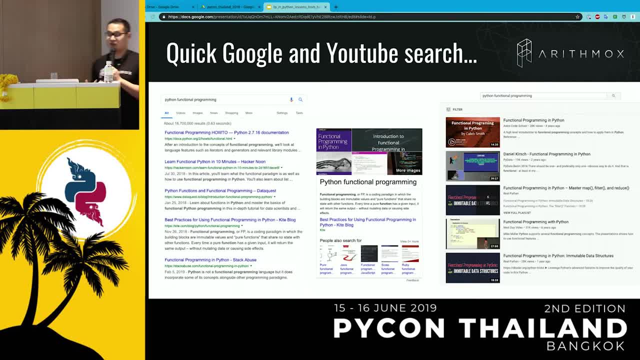 if you just do a quick Google or YouTube search on Python, functional programming, like you get so many hits and you think that Python is, you know there's actually something there- functional programming and Python- But you know if you really look at what they talk. 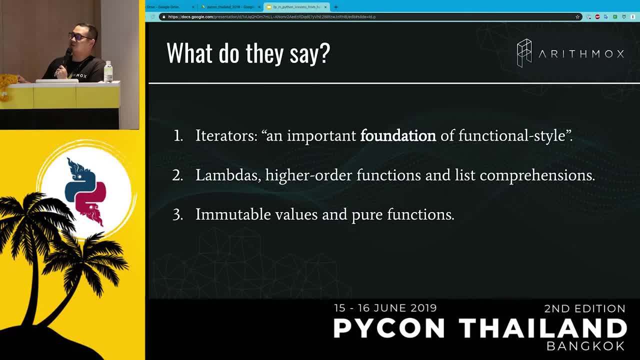 about. you know, a lot of them goes into iterators. I think that it's an important foundation of functional style. They get into these functional constructs of lambdas, higher order functions and less comprehensions. It's only in the third blog post that you get you know what I think is the real meat of functional programming. 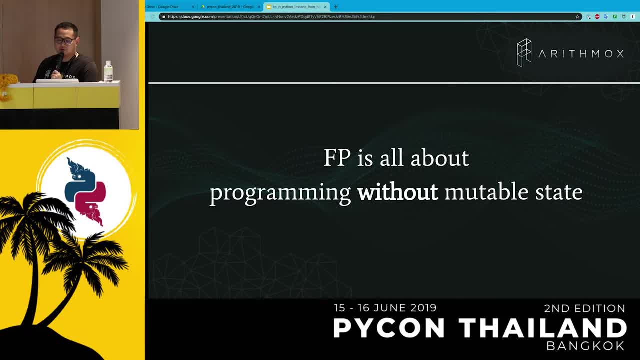 immutable values and pure functions. So for me, functional programming is all about programming without mutable state, right? You'd hear, perhaps intuitively, that functional programming is about programming with functions. Yeah, But it's not strictly correct, right? It's programming with. you know the way we define. 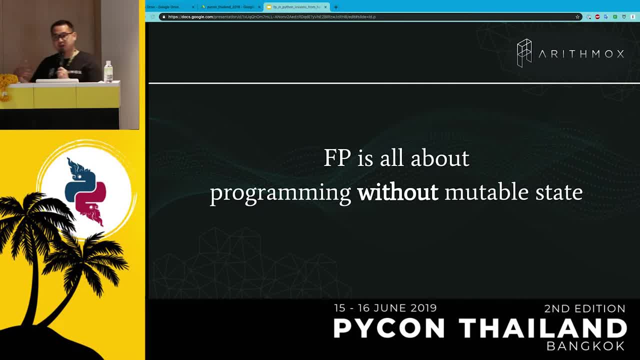 functions and Python is not exactly the same as functions in a mathematical sense, because within a function and Python you can actually grab like a global state and then modify something to it And you return something else in such a in a way that you know your output doesn't. 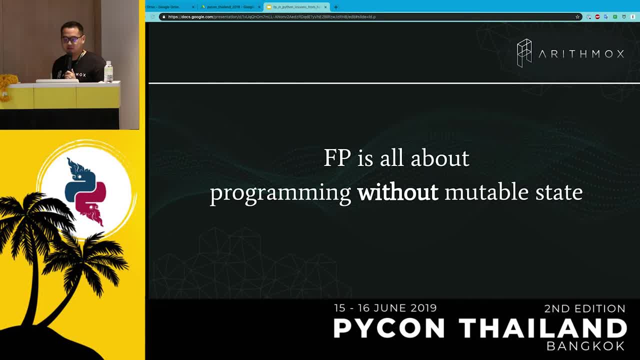 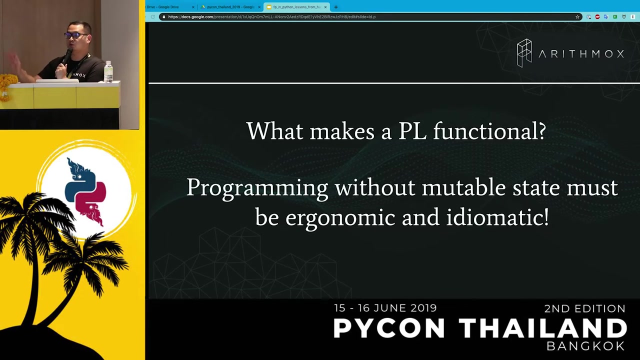 only depend on the inputs, So it's not a pure function, So it's not programming with functions. in that way, And if that's the line that we're going to take with functional programming, what is it that makes a programming language functional? And here I would argue that programming without mutable state must be one ergonomic. 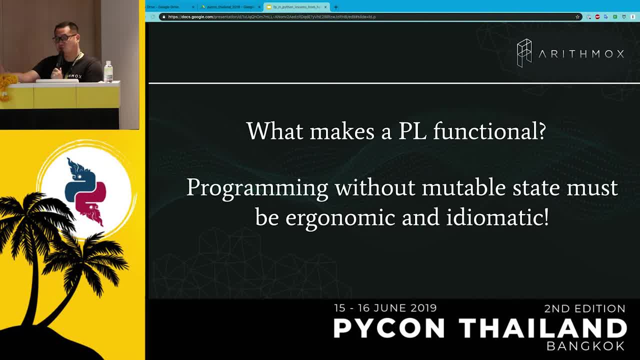 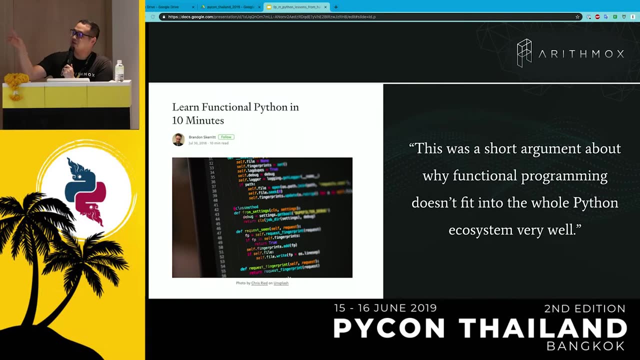 you're not fighting the language in order for you to do that And, secondly, it has to be idiomatic. Yeah, It's a style that is encouraged by the community that you should write your code in And, ironically, if you get, you know one of those blog posts that you found, there's something called learn. 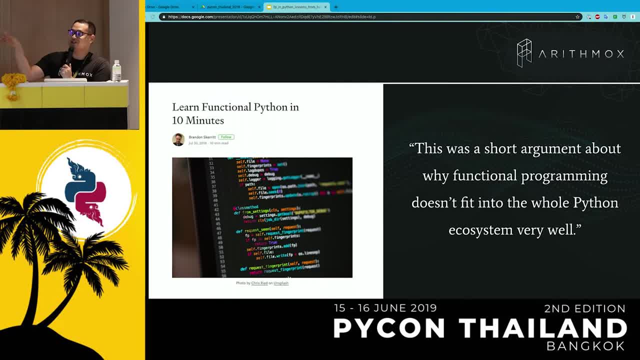 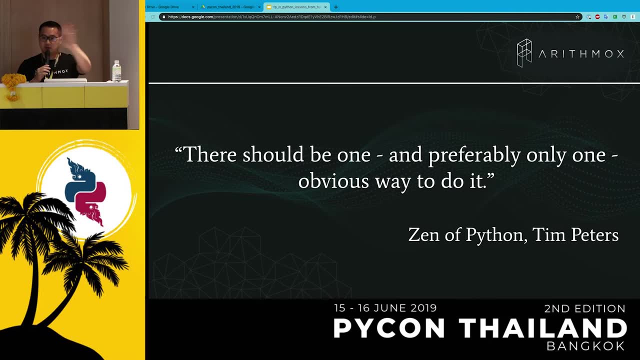 functional Python in 10 minutes. But inside there it's actually arguing that hey, functional programming doesn't fit the Python ecosystem very well. And here I think he correctly invokes that. you know one of the lines of the Zen of Python. you know if you do import. 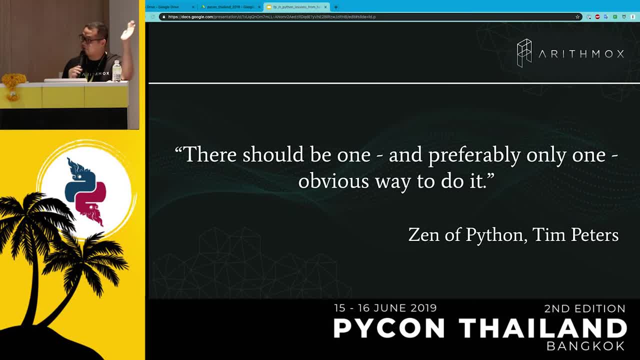 this in Python, one of the lines is that there should be one, and preferably only one, obvious way to do this, And if you look at the functional programming constructs that are useful for programming without states, you know sometimes it's not idiomatic in. 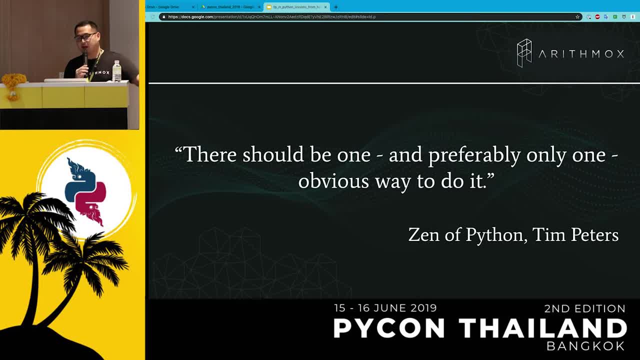 Python. you know I'm talking about higher order functions. People don't really use maps filters At some point. Guido wants to get rid of reduce partial and compose. You need to import and PEP 8 doesn't let you. 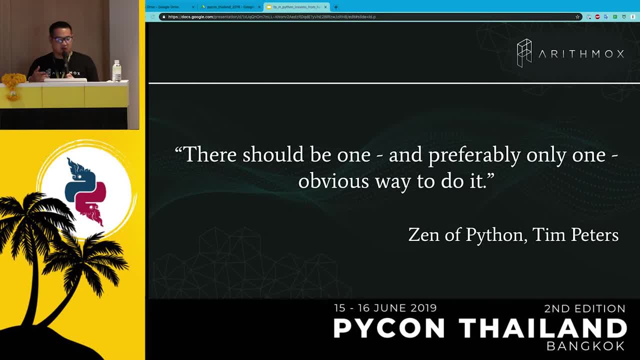 No, no, no, no, no, no, All right, fine, So this is a really Edu ange, All right. so we're going to go ahead and you do assigning lambda to a name you want to do. the def and recursion is a mess in. 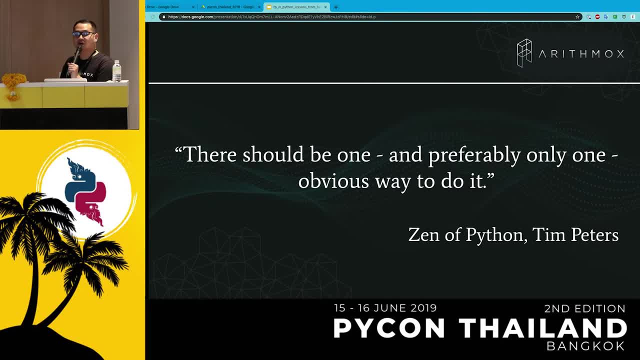 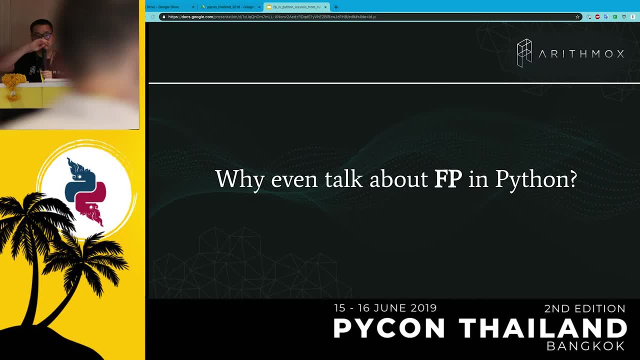 Python. So in some sense, maybe Python is not really a functional programming language. That's my argument. but why even talk about functional programming in Python, right? So I feel like I need to really preface this. I believe that you don't need to do all of those 100% immutable state. 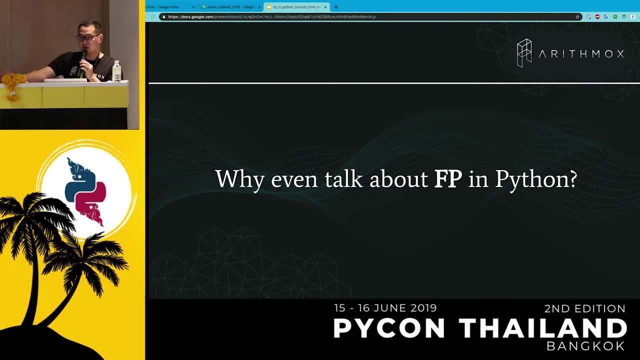 I think we can be very pragmatic here. take what we can, and I think there are still bigger lessons and concepts that we can port back. Sometimes side effects are okay. You don't need to be like Haskell. So I want to get the benefit of functional programming languages while staying with idiomatic. 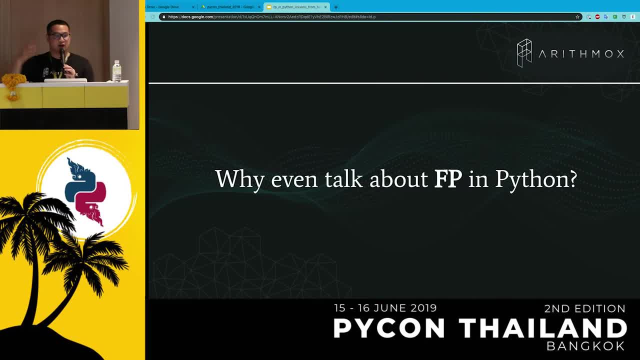 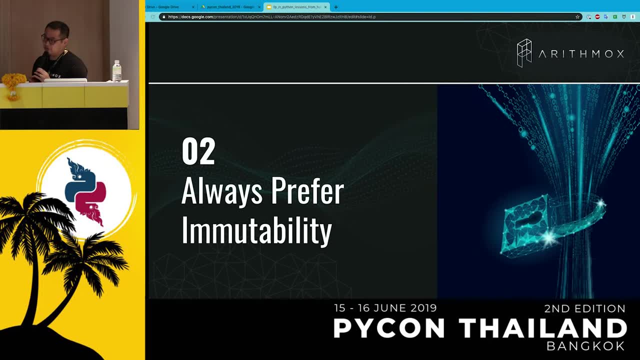 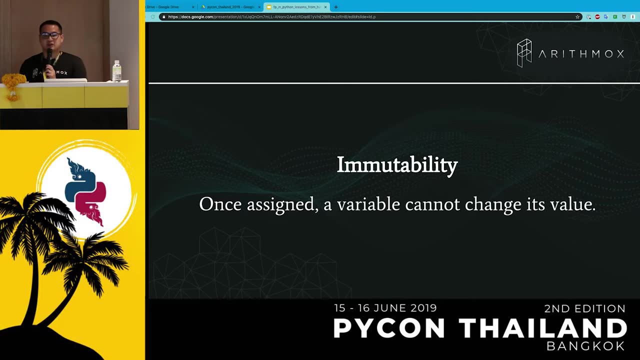 Python. So not necessarily writing these obscure higher-order languages, Not necessarily writing these obscure higher-order functions. With that in mind, I want to get to the very first thing about functional programming, and that's immutability. So immutability is this idea that once you assign a value, a variable shouldn't change. 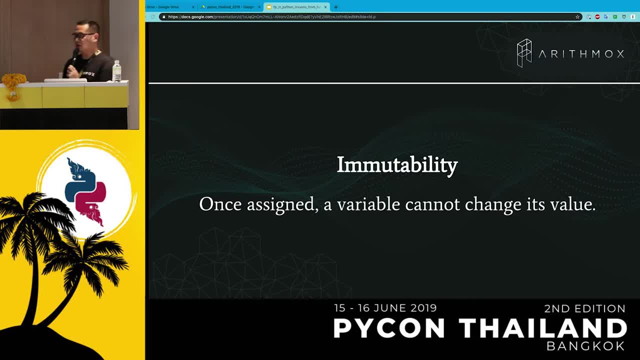 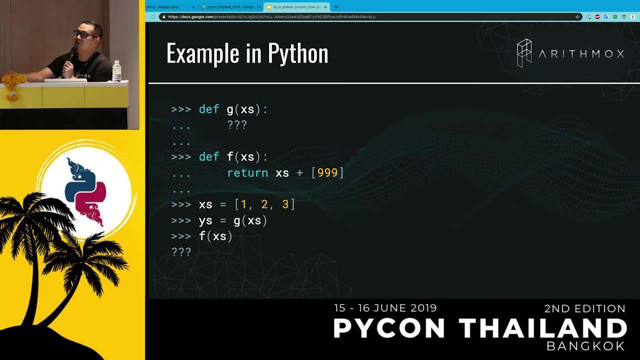 its value right And just looking at it like that, it's not maybe entirely clear what I'm saying. So I like to have an example. So this is an example in Python. So I have a function g. It could be somewhere else in the code base, so you're not exactly focusing on it, so you 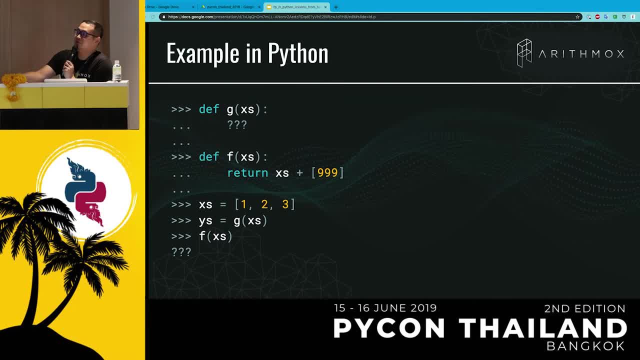 don't know what it actually does. And then you have a function f that presumably appends 999 to a list. So you declare your list xs 1,, 2,, 3, and then somewhere in there you apply g to xs. 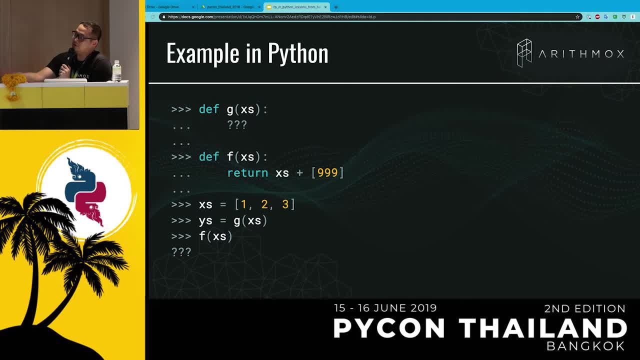 to get ys. Presumably, when you apply f to xs, you should get 1,, 2,, 3,, 999.. And then you apply g to xs to get ys. Presumably, when you apply f to xs, you should get 1,, 2,, 3,, 999. 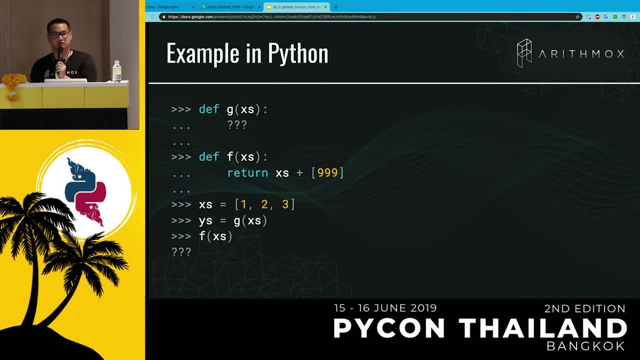 And then you apply g to xs to get ys. Do you think we can make that guarantee in Python? No, No right, Because you can be really doing something nasty with g, For instance. I can make a side effect here And then instead you get 3,, 2,, 1,, 999. 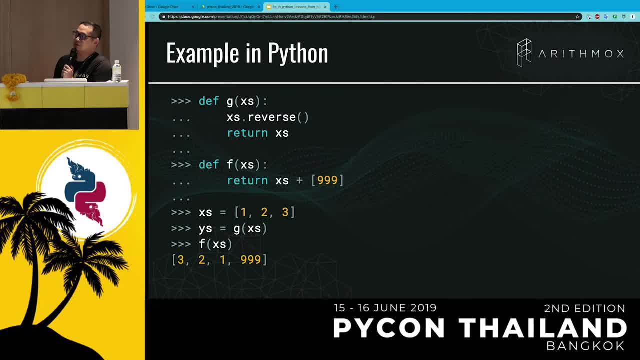 And if you think about that, there's another way to do this right. You'd think it'd be equivalent to do negative indexing, but it's not So. if you do reverse, it actually mutates that list, whereas if you do negative indexing. 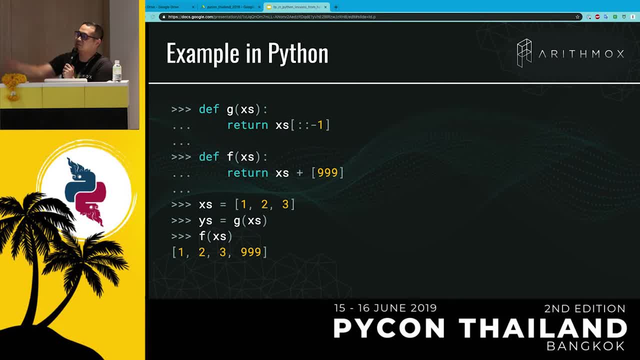 you actually make another copy of this, So there's performance consequences here, But then you do get a vastly different result. So here the list is mutable. I want to contrast this with what happens in Haskell. Same program in Haskell, right. 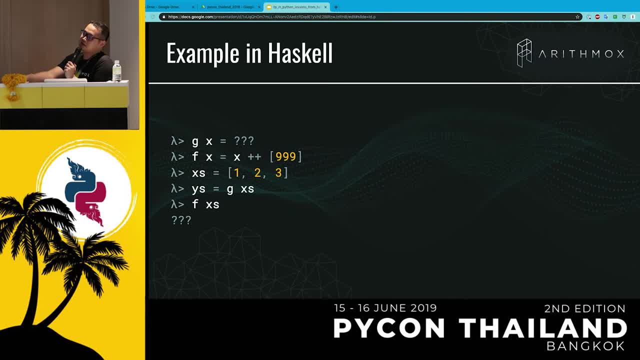 You get some g, you get some f, appending 999.. You've got some xs, and then here's ys applying g on xs, And actually in Haskell you can always, always guarantee that this is 1,, 2,, 3,, 999. 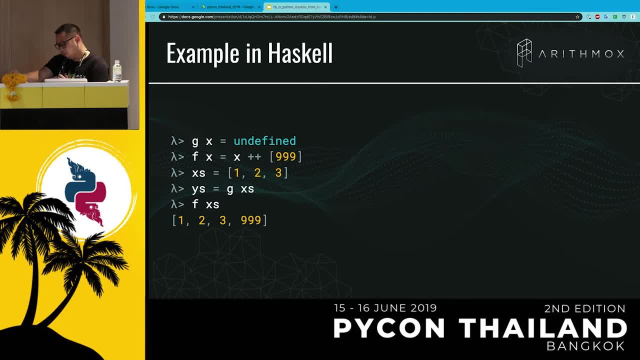 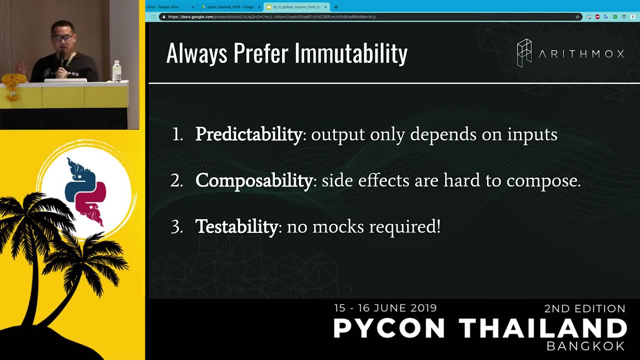 It doesn't matter what g is. This is because mutations or side effects is controlled by the type system in Haskell. We'll get into that in the next section, but this comes in very, very handy. Why is it handy? right Like there are a few benefits for you to writing this in an immutable way or immutable style. 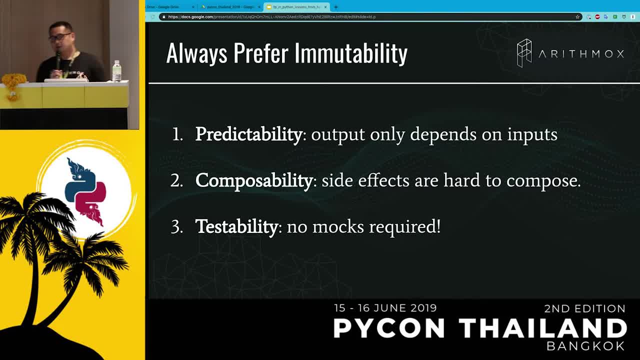 Firstly is predictability. You know people in the functional programming community like this. They're saying, oh, your code is easy to reason about. And really this is what they mean when they say it's easy to reason about. It's predictable. 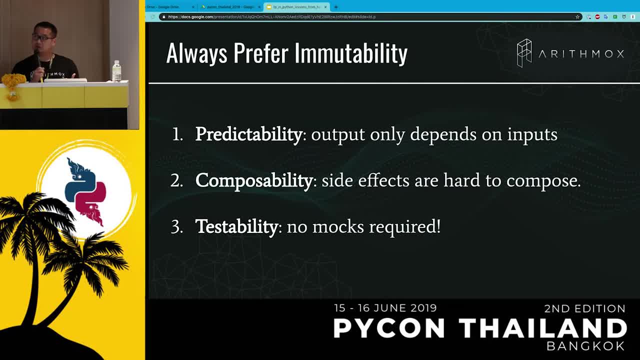 When you're looking at a function, your output depends only on the inputs, so that you don't necessarily have to look at other places in the code base to find out what exactly is happening there. And composability. So the name of the game in functional programming, when you want to build complex behaviors, is 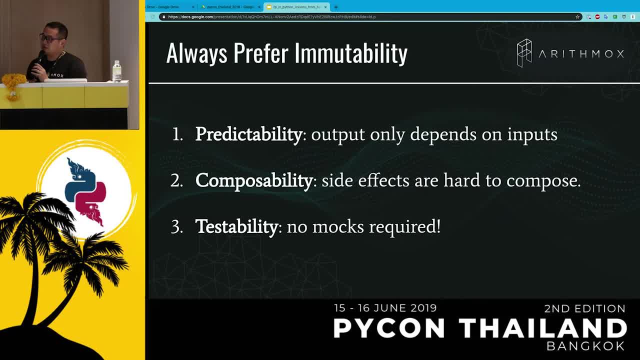 that you compose small functions together And you get complex functions. You get complex behavior by building on these small functions And it turns out that side effects is very, very hard to compose And if you put a side effect there you don't get this benefit. 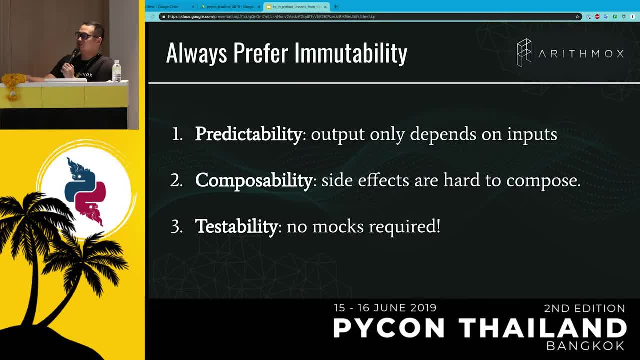 And finally, testability. I'm a huge fan of TDD. I hate it when I have to write mocks. It's just not fun to set up. So what does that mean in Python? How do we get this benefit in Python? 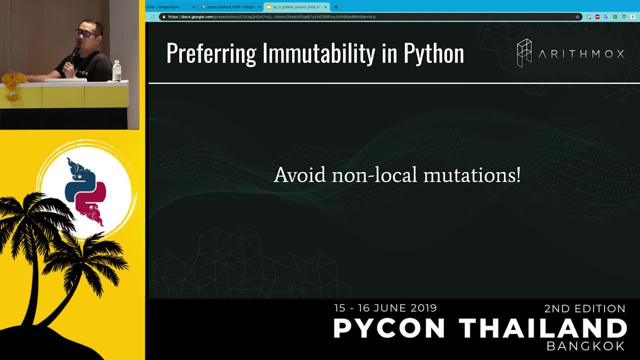 And I would argue, is that: avoid non-local mutations if you can help it. And what do I mean by that? Local stateful variables are OK. Say, you declare a stateful variable in a function and then you make a mutation. then and there. 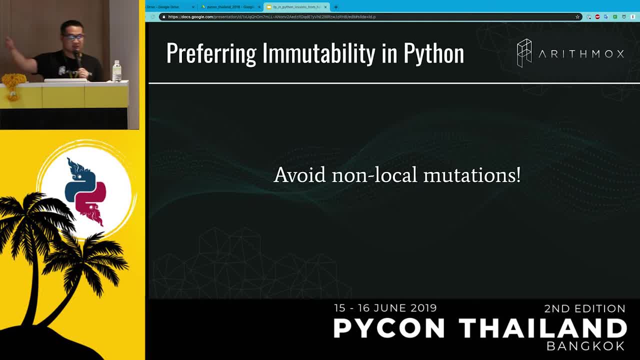 And then you return it, That function is still pure. This idea is captured with even in Haskell, Something called the strict threat monad, but it's not good there. The problem is, when you mutate that function, you can't do anything about it. 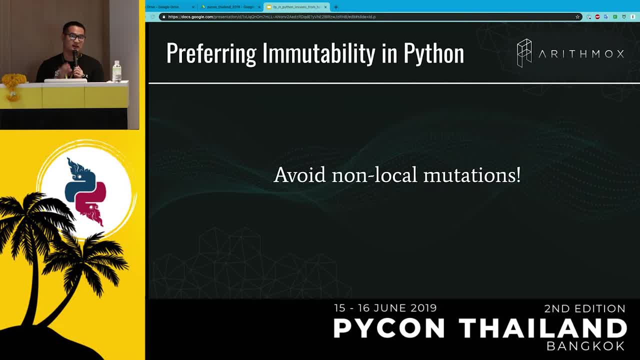 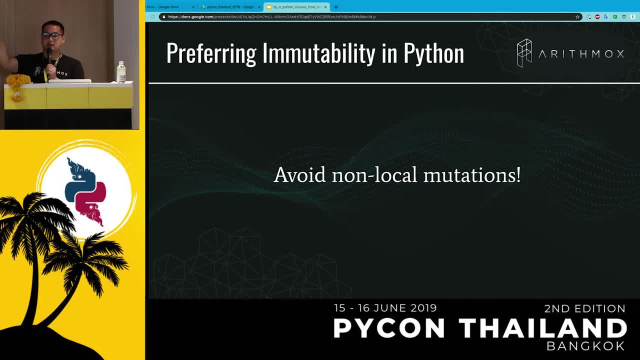 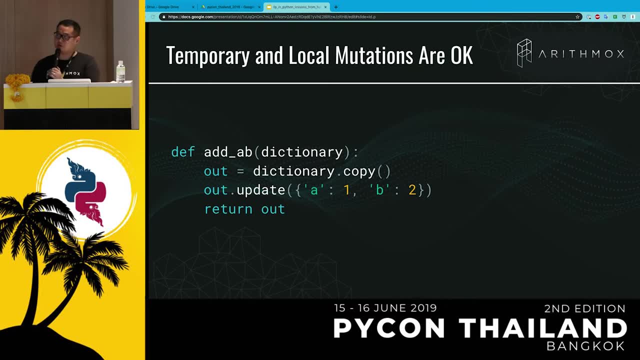 whenever that thing is mutated, someone has to keep track of what that mutation is, And that's hidden. So just to say, like, temporary local mutations are OK, So this is OK, right, Like I'm making a side effect, but it doesn't matter, right here? 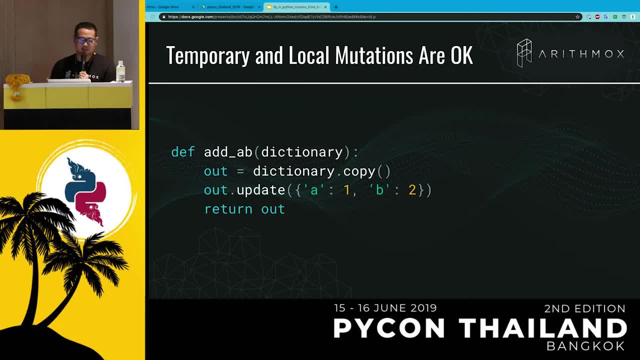 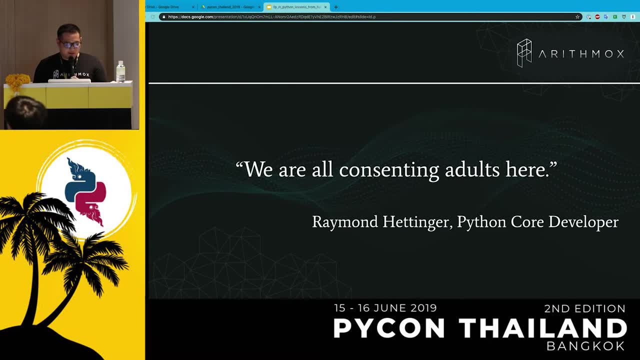 So this is what I'm alluding to. like you don't need to have this Haskell strictness every time, But you can still get the benefit. One of my favorite quotes in the Python community is that we're all consenting adults, Raymond Hadinger. actually, in the context of this is that when you're dealing with a third, 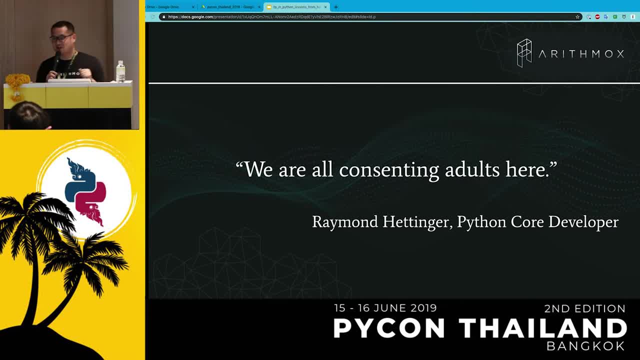 party classes. you don't go inside the internals and then change things there, because you don't know what you're going to be changing And to the same spirit, right like, whatever you're changing, then you're changing global state Like you don't want to do that. 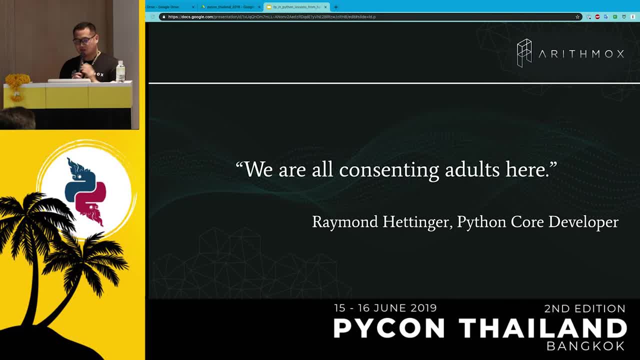 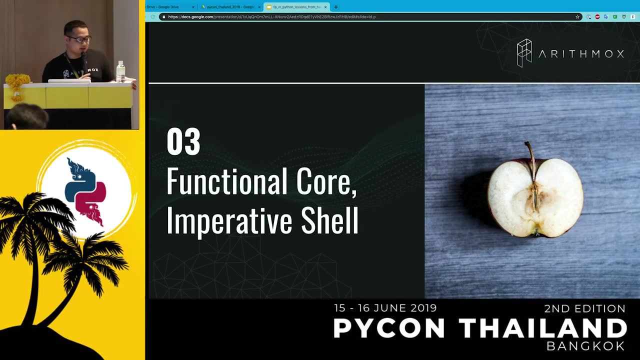 Like for me, consenting adults here mean: OK, let's, let's try to avoid that as much as possible. So don't make non-local mutations, That's, that's number one. So I want to go through the second point. Is there is anything not clear? 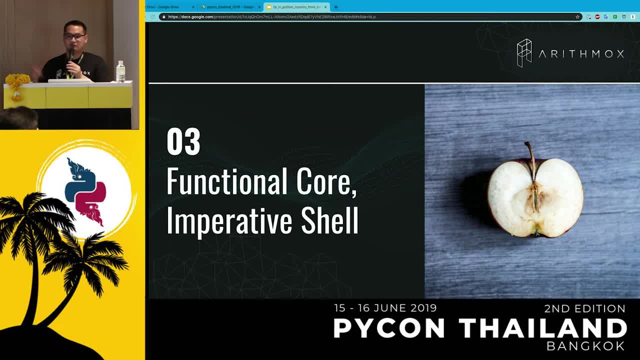 Is there any questions about immutability? OK, I think I hope that's clear. So the second thing I want to talk about As this idea of functional core and imperative shell. I'll get to it or what that means, but I want to take a detour to Haskell. 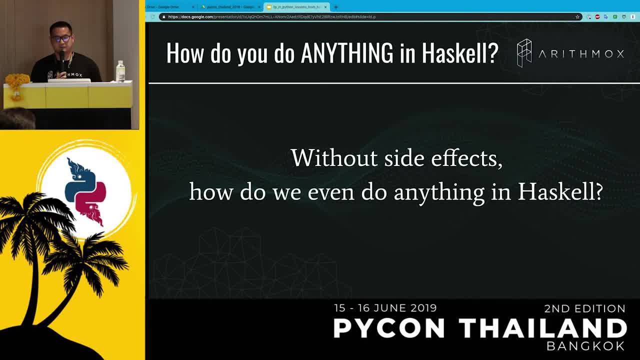 So I kind of left you hanging with Haskell, right. So I told you: OK, everything's pure, You can't make mutation, There are no side effects. But how do you even do anything useful in Haskell? Because if you need to print to standard out, that's a side effect. 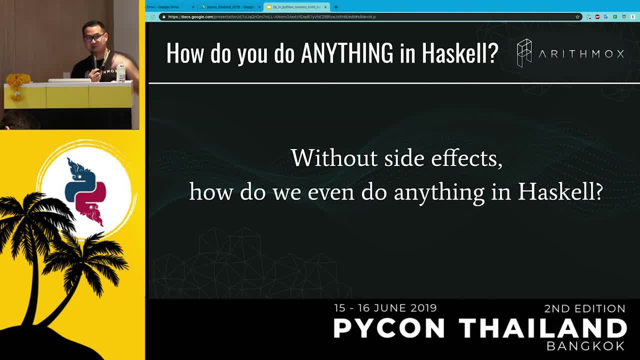 If you need to save to a file, that's a side effect. You need to send and receive requests. that's a side effect Like: how do you achieve this in Haskell, right? So there's something called the IO type, the input output type. 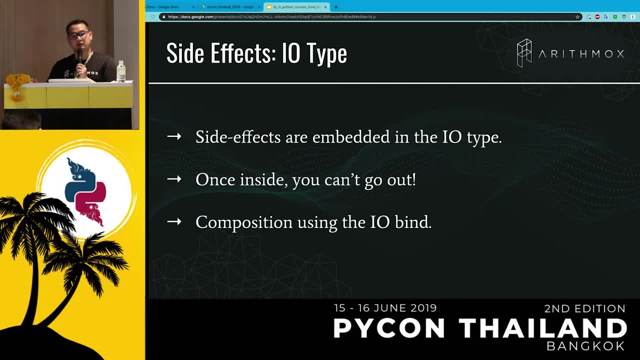 And really the side effects are controlled by Haskell's type system. And let me elaborate what I mean by this. An IO type Is: Is Does Takes a concrete type to make another concrete type Bear with me. So there's something called an IO of int. 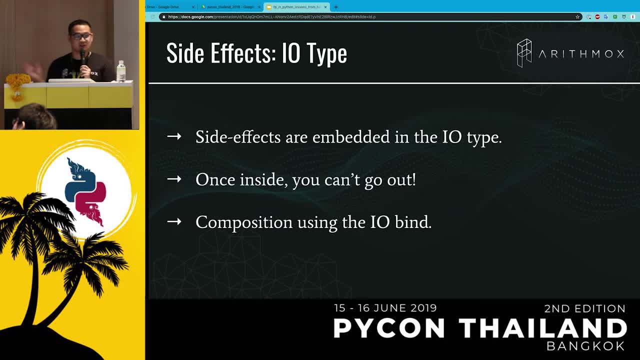 Just like there is a list of int. What is a list of int? A list of int is a list whose elements are integers. That's what a list of int is. A list itself is not a type. A list of int is a concrete type. 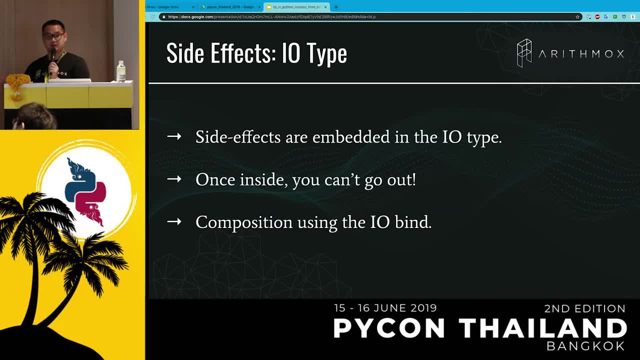 An IO is not really a type. There's not a complete type, but there's an IO of int. So what does it mean to have an IO of int? IO of 1 means that you arrive at this value of 1 using some sort of a side. 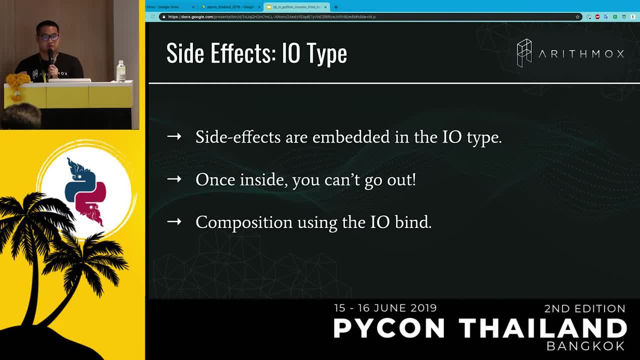 effect or stateful computation. So I can have an IO of 2, same thing: 2 is just a number, but I arrive at that number 2 based on a side effect. So I can change this thing. So I can plus 2 to a 1 to get a 3, but if I have an IO of 1, you cannot. 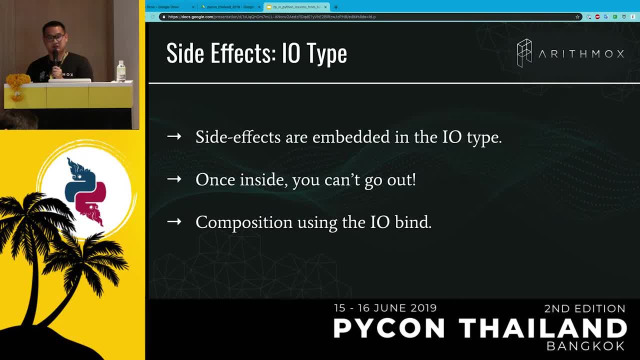 get out. The type system doesn't let you to get out, So you can get an IO of 3 from IO of 1, right? Because well, if you arrive to 1 using a side effect, you cannot arrive to a 3 using something pure, Like. once you're in, you cannot get. 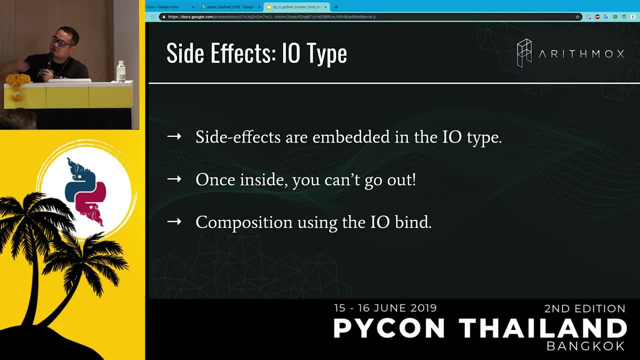 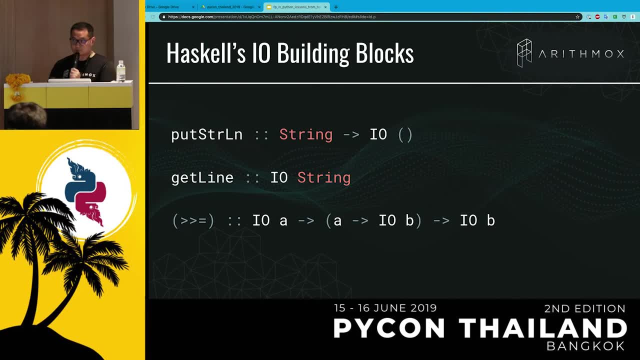 out And you can combine these functions together using what's called the IO bind. Some examples just to crystallize this clearly. Putsterlin is a print function in Haskell. It takes on a string and it gives you an IO of nothing. So think about it. This is like a print function in Python, right? 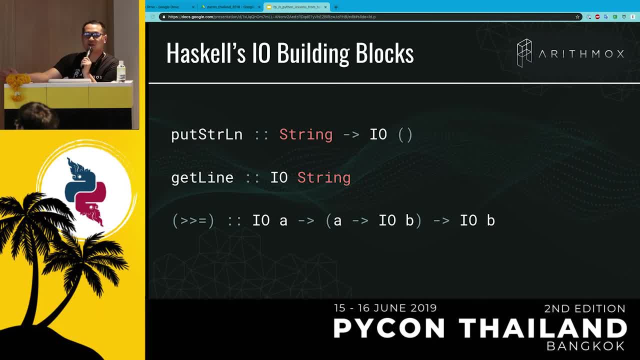 It takes on a string, It gives you none, It gives you nothing. But here you have to mark that side effect that you've written to standard out with an IO. So it's an IO of nothing. Get line is a bit like input in Python. It gives you. 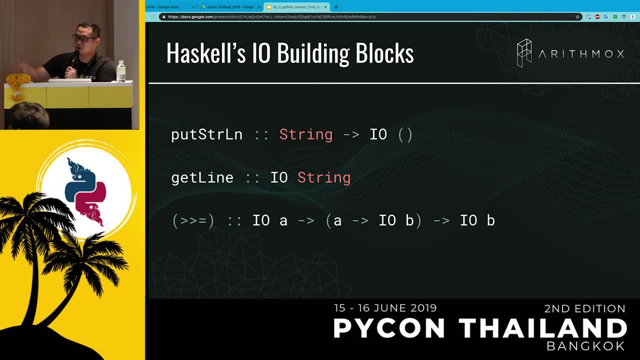 an IO of string Because it's a side effect. People write something. You cannot control that as a pure computation. That's an IO of string. The last thing is what's called the IO bind. But that's how? say, you've got an IO of 1, you want to change it to IO of 3, that's. 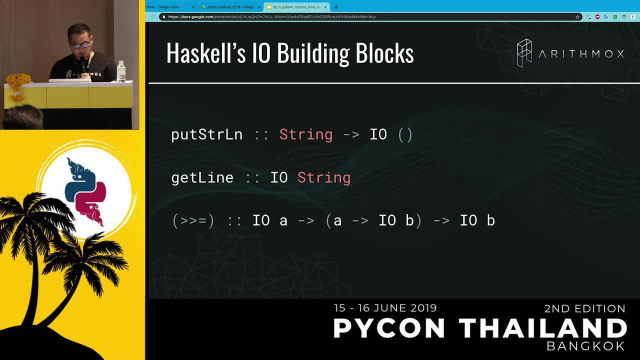 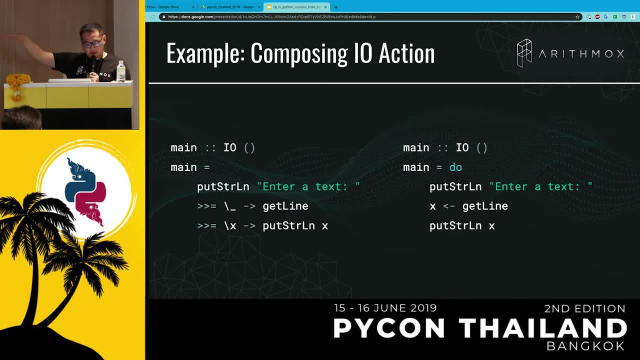 how you do it, Or IO of like a string of 1 or whatever. So that's going a bit deep, right, But this is a program that you can write that basically prints: enter a text, you give it back something and then it'll just print it back. Excuse me So. 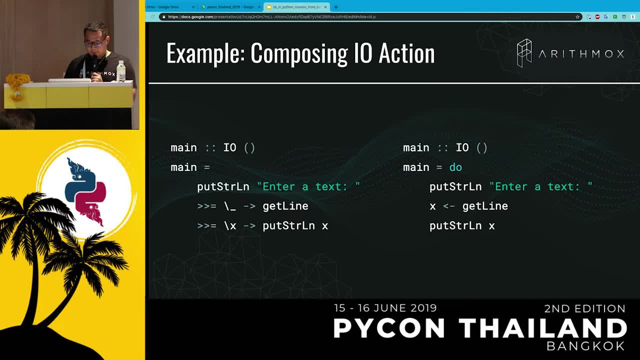 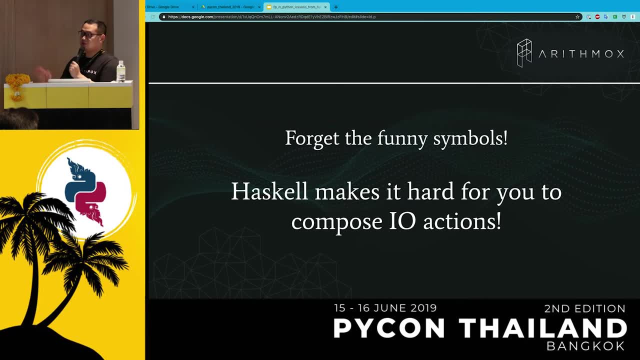 these two things are equivalent, And the point that I want to make here is that forget the funny symbols. They don't matter, They really do not matter. But Haskell makes it hard for you to compose IO actions Once you have a side effect. 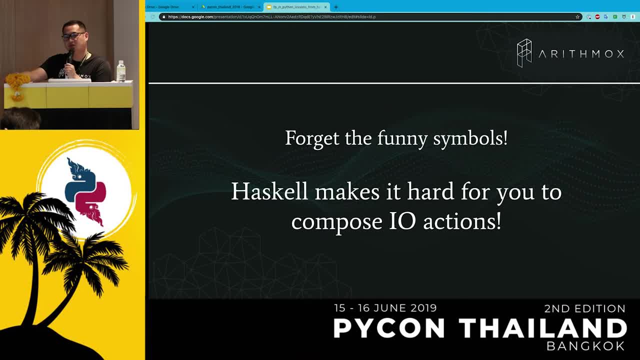 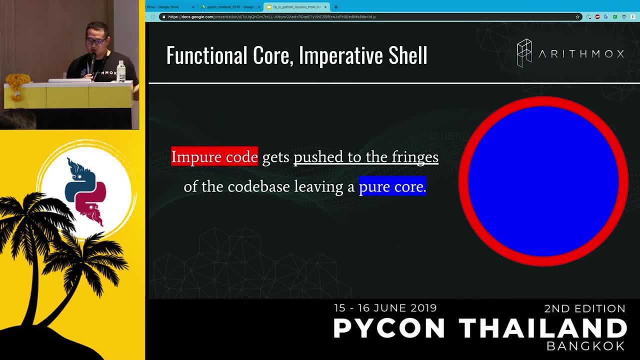 there like you're making your life very, very hard to do the next thing. It's not as natural. So they end up having this idea of pure inside. But then the imperative- like the stuff that you really have to make a side effect is a thin layer of your application. So you push. 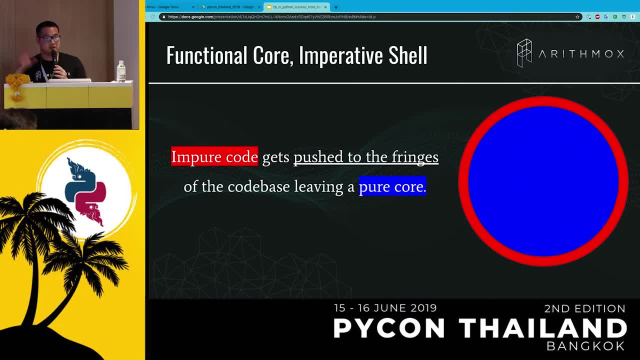 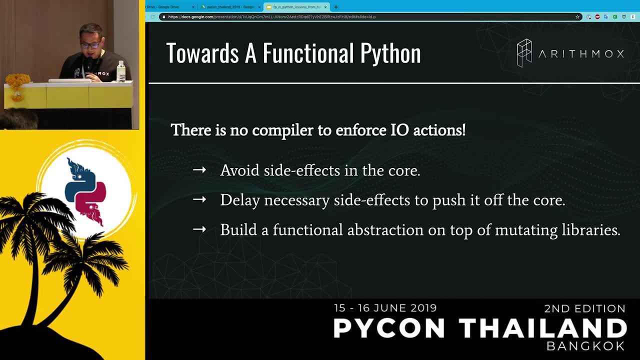 out these impure code to the fringes of the code base so that what's inside is pure, What's inside is just immutable stuff. And we can do this in Python, right, There isn't a compiler to say, hey, you did it wrong. 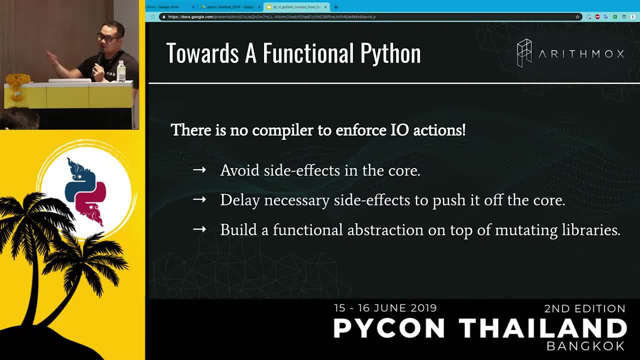 You can rely on your own discipline to say, hey, you know this is the core logic, So maybe I shouldn't be doing the side effects there. So you can always delay the necessary side effects to push it off the core. You do it at the end And sometimes you know we use Python. 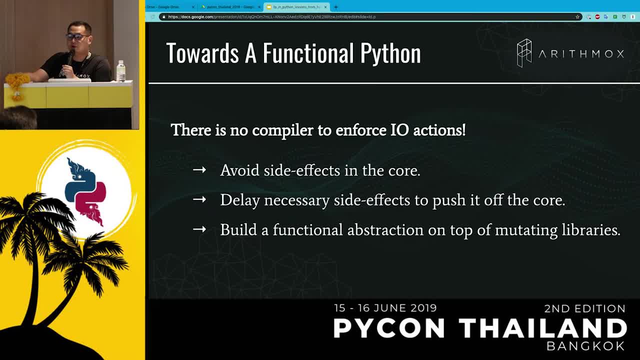 partly because it has a really good third party ecosystem right And sometimes they're very muted mutating. So what you can do is build a functional abstraction such that you only deal with your own thing, which is nice and immutable, and then do the mutation. 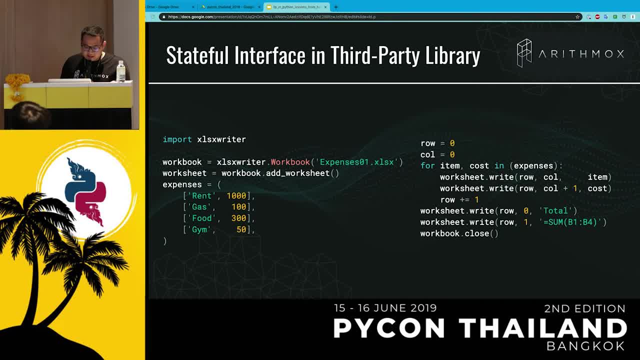 right at the end. I'll give you an example. So recently I had to deal with this library called xlsxwriter. It basically just writes spreadsheets for you. So this small little code here basically is just: it makes a workbook. You grab the worksheet And then you write this label and value to: 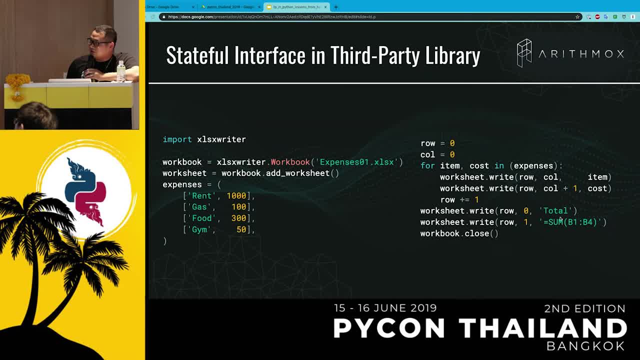 the row and column that you like. You can even write a string or a formula. Then you close it and you're done. It's like a very simple spreadsheet Problems. All of these stuff are side effects And, as you can see, if you think of this as 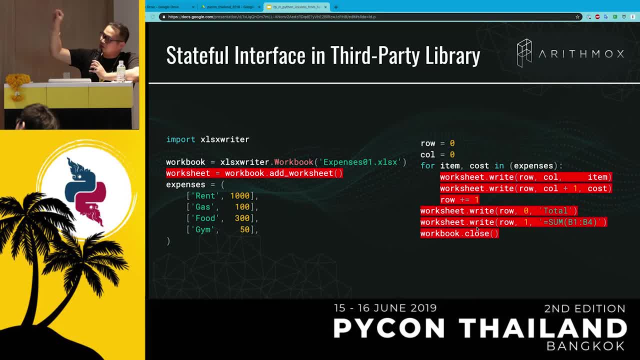 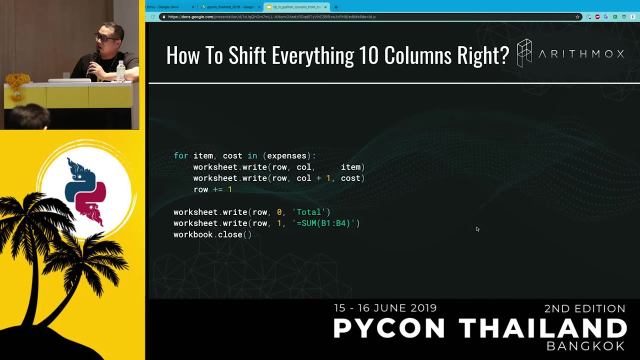 the entire application. you don't have a functional core. These things are inside the core. So you have an imperative core And it looks like it's not a problem. It's easy enough to understand. But the problem is that what if I want to shift everything 10 columns to the right? Presumably you can. 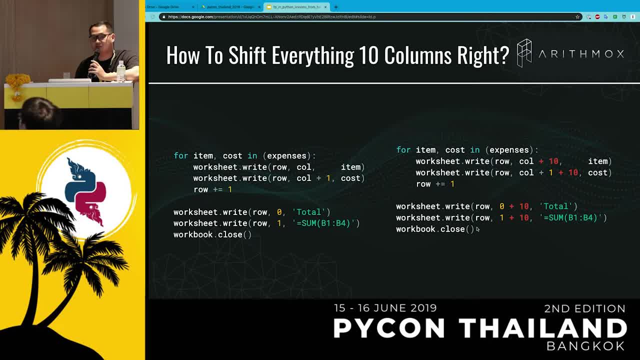 do this Again. it's simple enough. You just put plus 10 to everything. But this seems wrong, right? This seems wrong because, well, you're dealing with the business logic there. You're putting your labels, your values there. why does shifting it 10 places there has anything to do with it, and why does it? 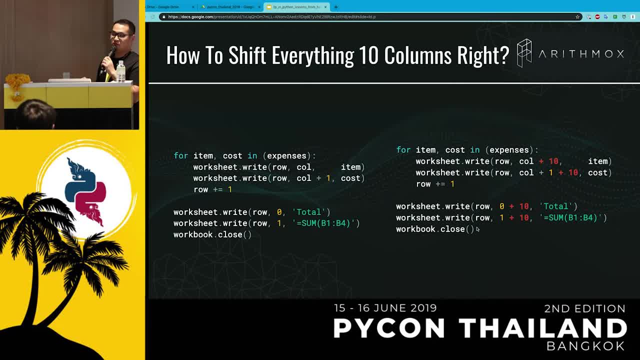 have to be conflated inside the business core. that makes sense. it should just be a simple modification of the code. i just, you know, i made this thing. oh, stops working. there's another one here, test, test, okay, so it stops working. uh, yeah, sorry, yeah, excuse me. um, so you, you did all the. 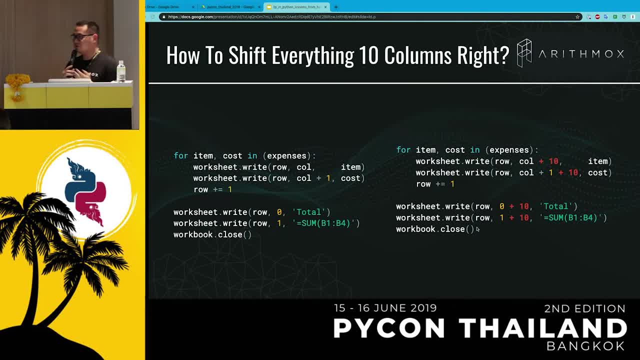 logic there. you just want to shift it to the right, and that should be easy, whereas this you kind of you kind of have to get into the forest a little bit and then, like, find where you have to input it and there's replication as well. this is what i mean by saying side effects. side effects are hard. 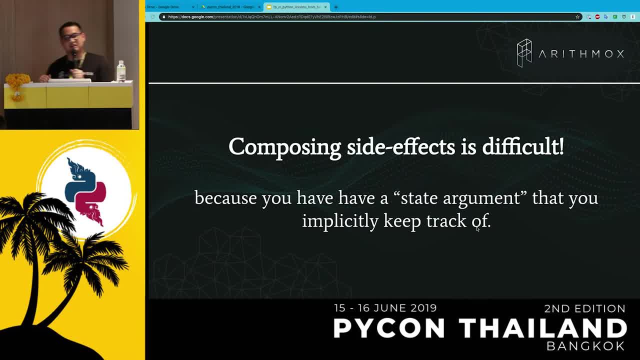 to compose uh, because essentially you have this state argument. that's implicit. it's not there in the arguments list, but the global state is actually part of your uh. it's part of your argument and this is like a just a very simple fix that you could do. it's like it's just a. 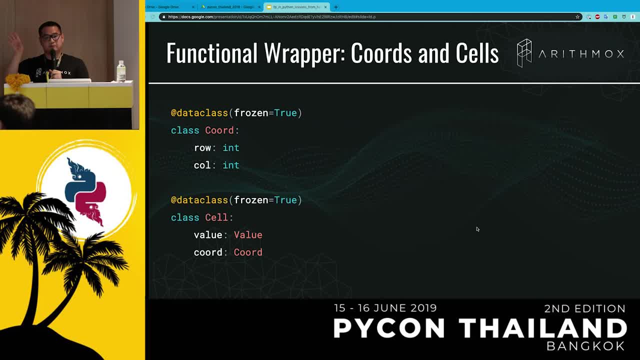 functional wrapper. really, the important thing is that you want to put, you want to write where at a coordinate, and then there's a cell which just takes in a value and a coordinate and and this is immutable, right like this. it's just numbers and you can also have a function that. 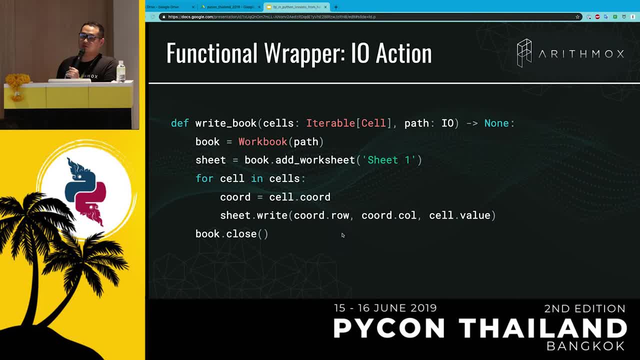 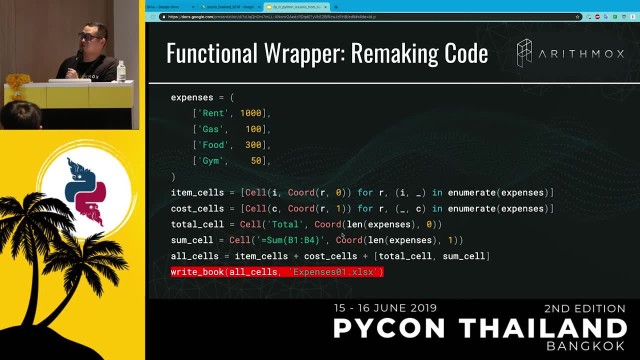 just takes in all the cells and then write it in one go. um, if we do this, i can rewrite that thing to look like this: uh, so i, i accumulate all the cells in one go, um, i've got the items, cost, totals or whatever, and then i, i put everything together and then i make the right, uh. 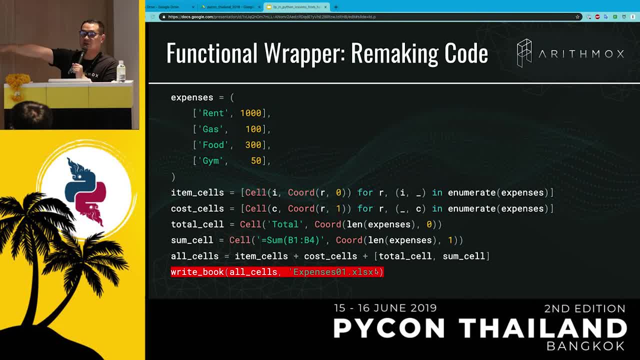 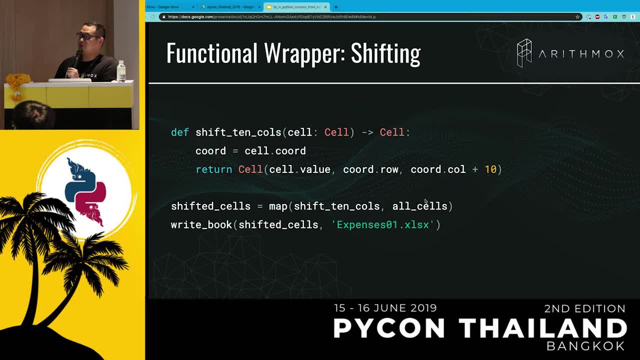 there. so that's the edge of my application: only at the very end. why does this make sense? well, if i want to shift everything to the right, i can reuse this: all cells, like i don't change anything from the logic, like it's one. you're one composition away and then everything else stays the same. 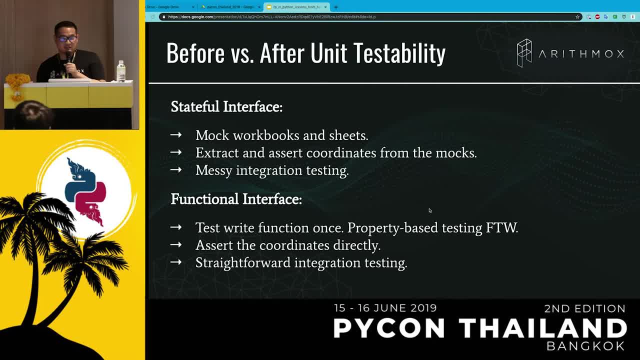 so that's kind of the idea, it's. it's, it's nicer to test as well again, uh, no mocks. uh, because you know you're just looking at the cells and the coordinates, they're just there. um, integration testing like this is easy enough, but what if you're? you have like 10 sheets and 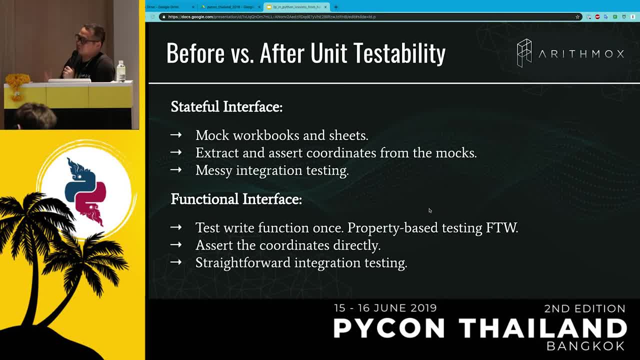 then 100 books, uh, like how you know, you want to make sure everything goes together, whereas they're just values. they're just there, um, and i think after this talk there's property based testing. uh, that's something that you can write that goes very well with functional programming. 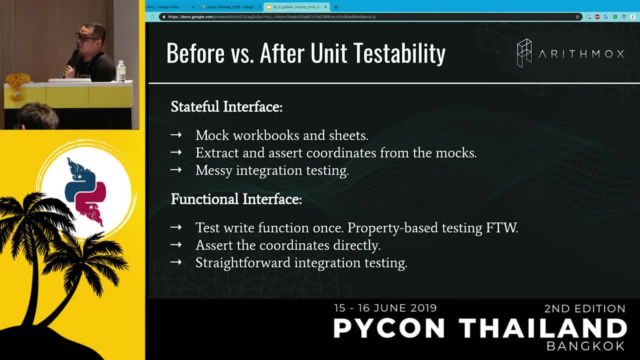 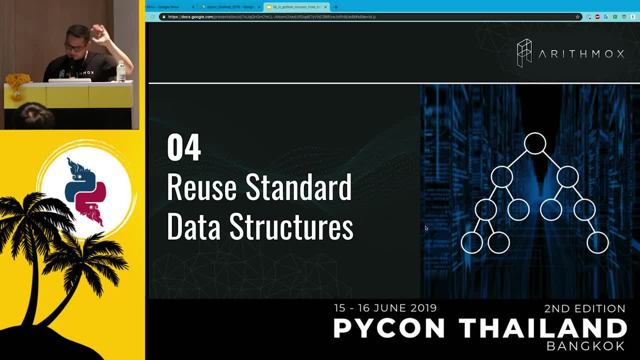 that's, that's awesome. um, yeah, so this is my case for functional core but imperative shell. that's the entire series on immutability and how to structure your program. i want to change to something um a bit different now. um, so, i'm newish to closure um this. so, uh, please correct me if i. 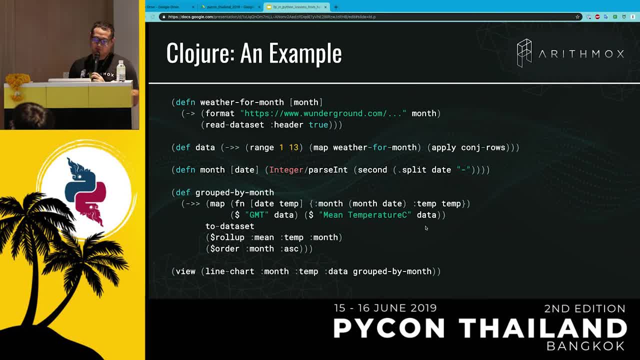 make any mistake. um, so this would be a lesson from cruiser. um so, just an example code. it doesn't matter what it says. uh, i took this from encounter, which is the data science and stats library for a. uh, it's a lisp right. uh, so that means you work directly with the abstract syntax tree. 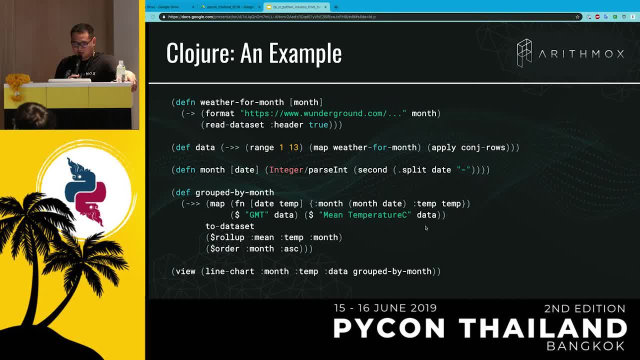 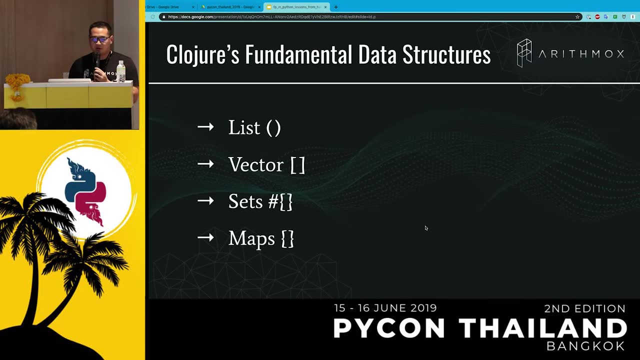 uh, it has all the really nice parentheses. uh, you don't see any types, so it's dynamically typed. um. so what's so special about this language, right? what? what kind of lesson can we draw from it for our python code? so one remarkable thing about closure is that, even though it runs on the jvm. 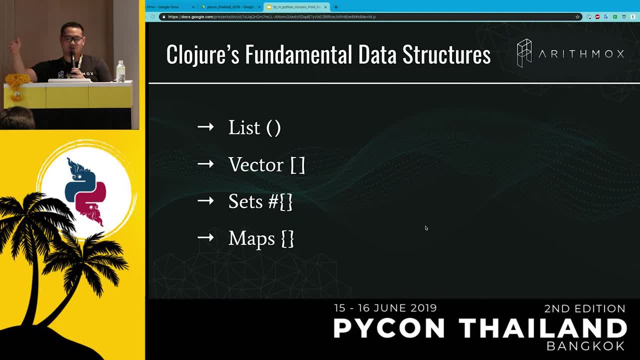 and you have all the powers and all the object oriented glory of java. idiomatic closure encourages you to use this. you know fundamental uh data structures so people typically use you know as a default list, vector sets and maps. like they don't create class on top of a class on top. 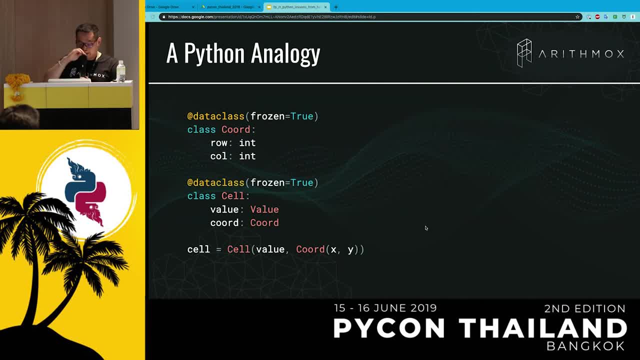 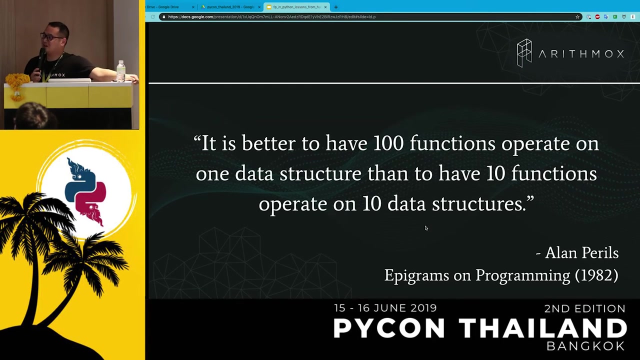 of class on top of class. so a python analogy: uh, we did this, uh, before. uh, it's as if, like okay, like forget, forget this, like we're just going to do this, like uh, yeah, um, but why? right? so it's very hard to read a closure tutorial without coming across this quote. it's alan perlis who's the. 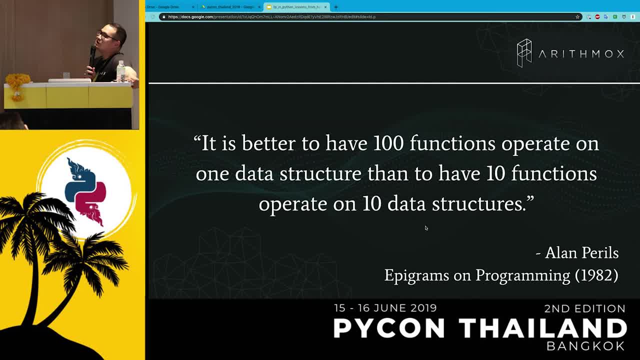 one of the pioneers of computers right computer science. it is better to have 100 functions operating on one data structure rather than having 10 functions operating on 10 data structures, and this is a statement about composability right, like if you have 100 functions operating on one. 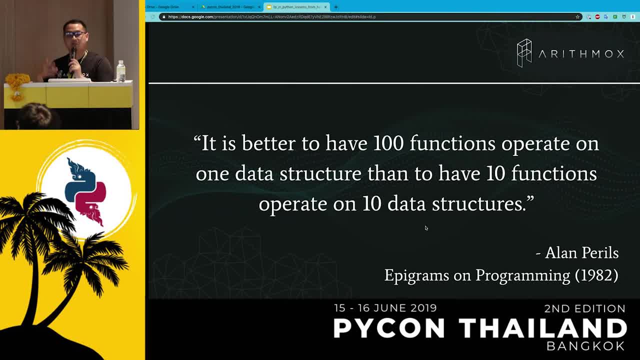 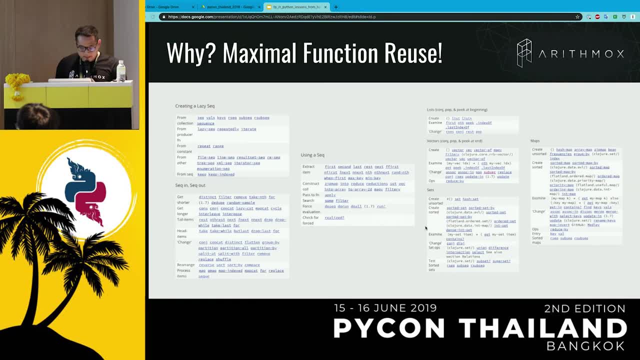 data structure. you can arbitrarily compose them together so that you can make complex behaviors using small pieces that are tractable for you. and closure has this wonderful uh functions that are there already. you can't really see this, but these are the functions for lists, vectors, maps, so this: 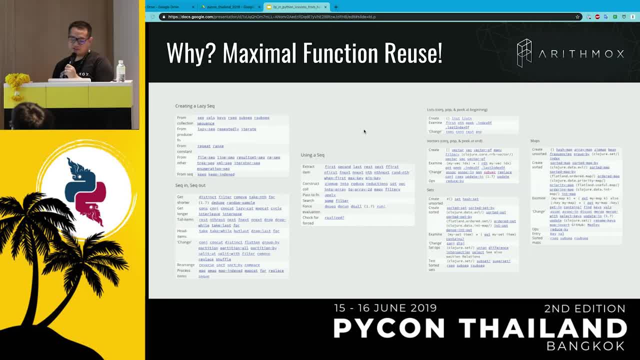 is a closure cheat sheet and they have what something called the sequence protocol. so these are functions that work on all these fundamental data structures, um, arbitrarily and agnostically. so it doesn't really care what that thing is. you can always get the first, second, last, rest next and first on all these stuff. 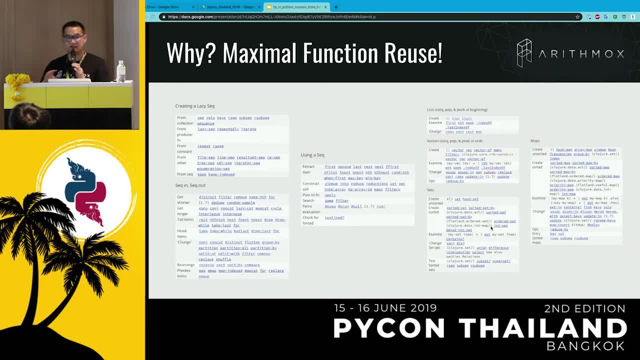 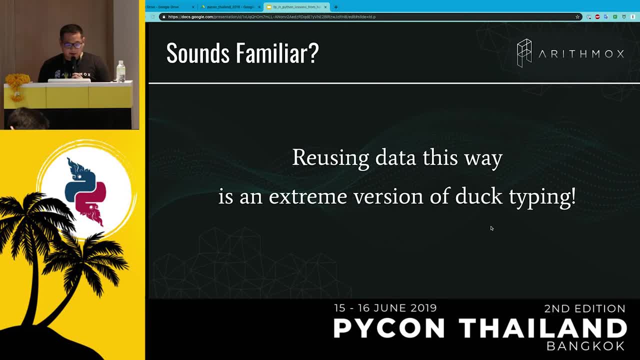 and yeah, it goes back to composition, right, if you have all these things, that's enough for you to compose them together and you don't need, uh, anything new. and i argue that you know this should sound somewhat familiar for uh, for us python users, right, because in some ways it's like kind of a duck typing, right, it's uh if it walks like a duck. 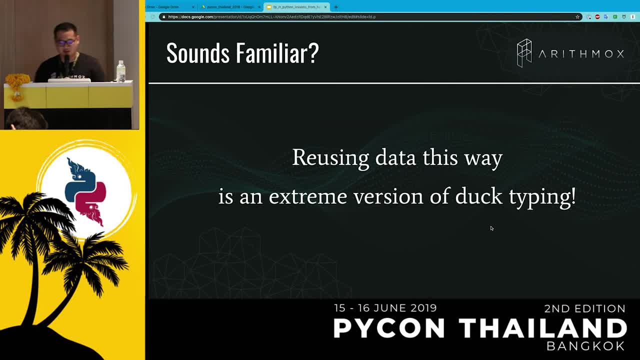 it quacks like a duck. uh, i'll treat it as a duck. and you know, if you give me a dictionary, it has a row and column on it. i'll treat it like a coordinate. and if you have, you give me a value and a coordinate, i'll treat it like a cell. so as long as it satisfies these conditions, so you know. 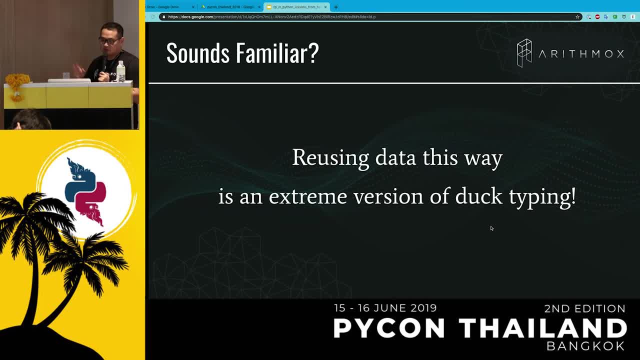 um, you know i'm going to treat it in a particular way, so that's doable in python, but it seems a bit sloppy, right, like you've got like this nested dictionaries and all that. like it seems sloppy. it seems like you're you're missing something, um, and yeah, i mean we do lose something, right, we we? 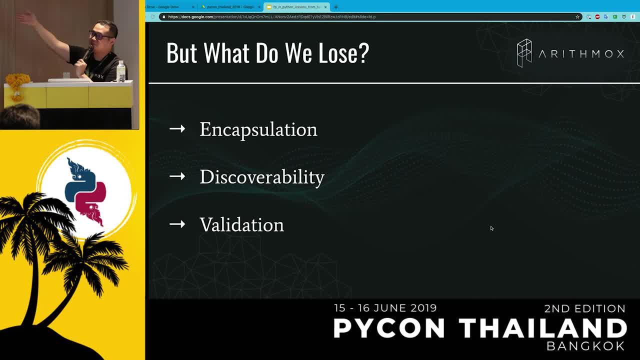 firstly, we lose encapsulation because you know you, you can say that this is a port in it and, uh, maybe you can have like helper methods, that, uh, that you know, maybe it shifts itself or whatever, um, and you don't have to really worry about the internals of what, what actually is there, everything just works. whereas with the 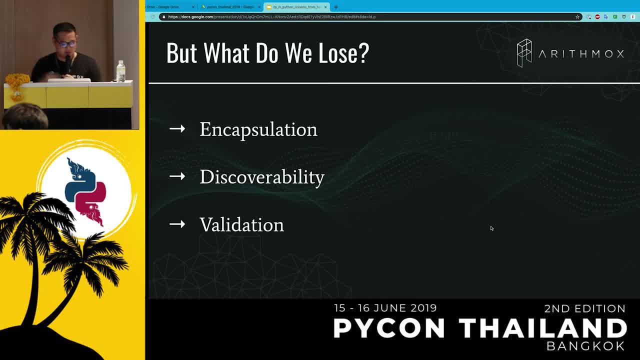 with the dictionary. it's like you're exposing yourself to everything. um, and discoverability, uh, you know this is the point of like static methods, right, um, you know, people put related methods together in a class and if it's just a dictionary like, you don't have these methods. 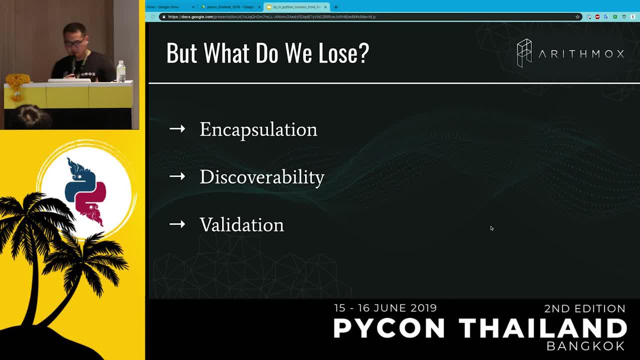 it's nice to know. like you know, these are sometimes bundled together, but they can't be now. so closure's answer for like these two problems is like having well-defined, uh, well-structured namespaces. so it really goes back to the programmer's discipline to put stuff in the 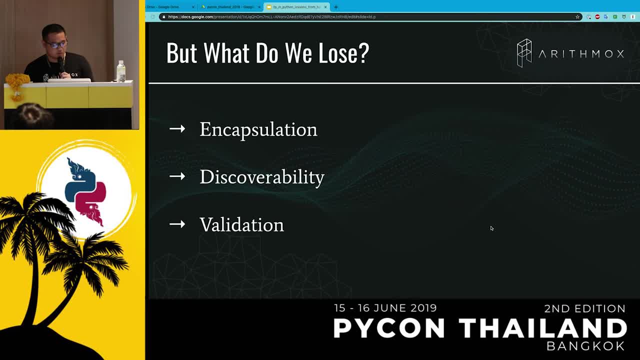 right namespaces, and then you're, you're, you know, you know where to find stuff. and i want to deep down a little bit on the this idea of validation, though i think this is the interesting part, something that we, you know, can actually change the way we write python. um, you lose the very little validation you have left. 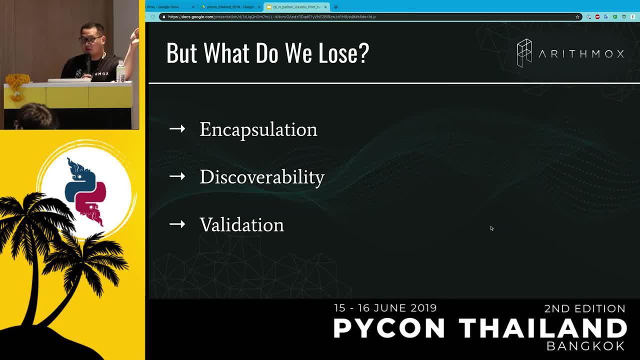 in a dynamically typed python, right. so maybe you can have a coordinate, you can put zero and one there, but you can't. you know you can't instantiate something without a column, let's say. but you can always instantiate an empty dictionary. so if you represent a coordinate as a dictionary, you don't. 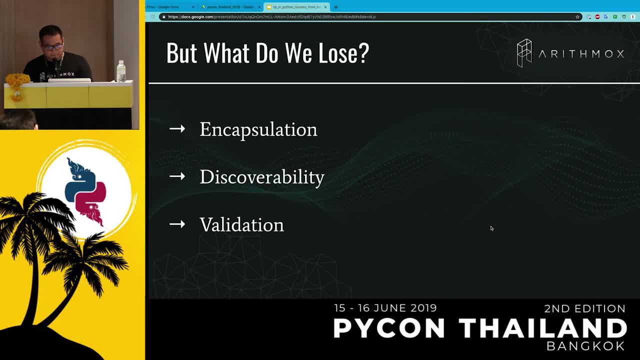 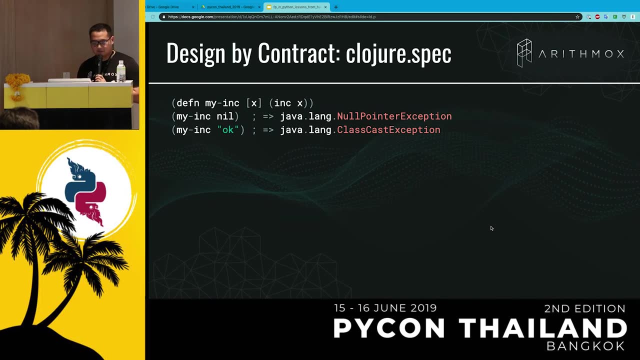 get this check um. it's a very nice technique that i feel is underused in python, but it's really gaining some grounds and closure. and that's designed by contract. um. designed by contract is basically a bunch of asserts of pre-conditions and post conditions, but structured in a nice way i'll give. 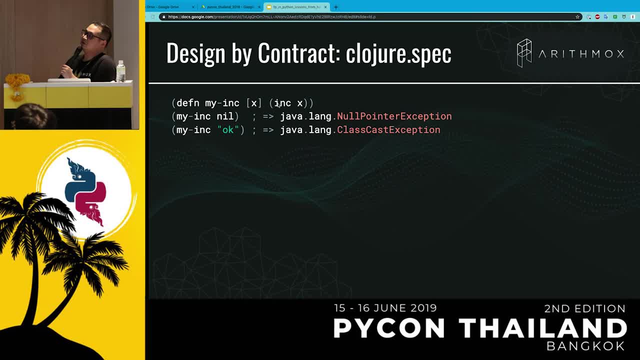 you an example. so this is a function declaration that just increments something by one right and it's: uh, presumably it takes a number, so that if you give you give it anything else, you get these unuseful errors, but you can spec it. so there's a library called closure spec. 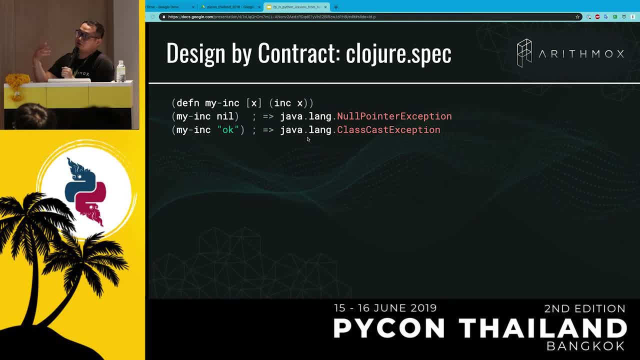 that allows to you, that allows you to um give it some contracts. so these are pre preconditions and post conditions, as an example. so this is a spec for uh for my function. look, the arguments have to be a number and the return has to be a number. that's all it's saying. 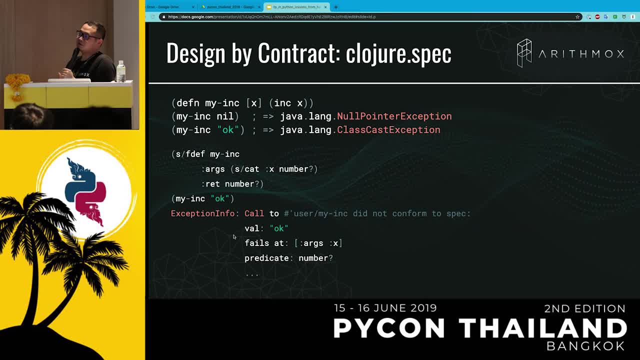 so that when you call it with a string you get this nicer exception. it says: look, hey you. you told me that it's going to be a number, but it's not. so, uh, it did not conform to spec. it's nothing else than an insert that has a nice. 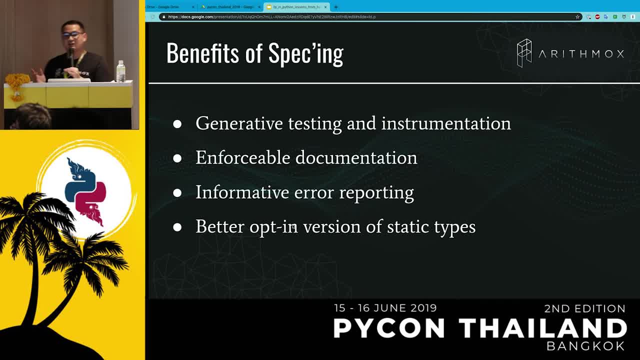 error message to it and the idea is that look, hey, uh, you get things for free if you do this in closure, specifically, if you spec something, you get this generative testing for free. so this idea of property based testing, so you can generate a test example or test cases automatically and then you can check whether or not it conforms to. 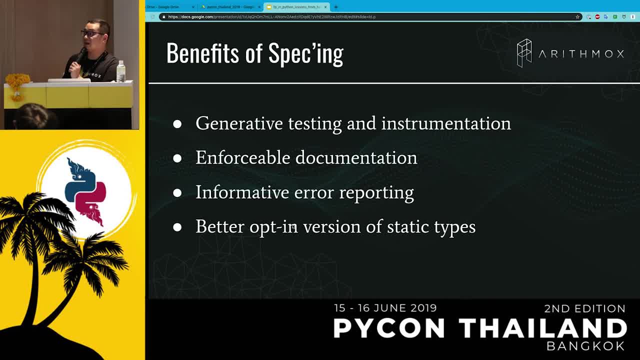 the, the function that you actually wrote. it can also act as enforceable documentation, informative error reporting, and there's nothing stopping you from using the contracts to just define types. but then you can do it better, like, say, you want to have a list of just numbers, but the list has to- uh, the length has to be bigger than six. try doing that in haskell. you can't. 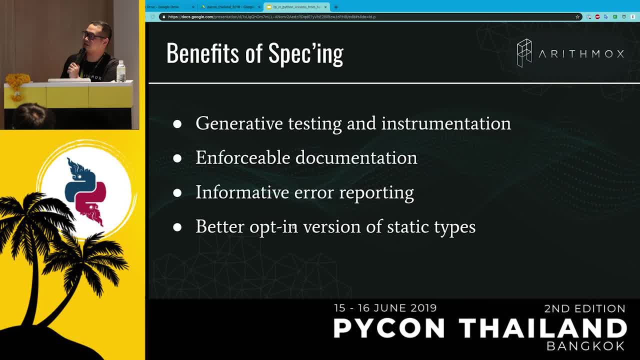 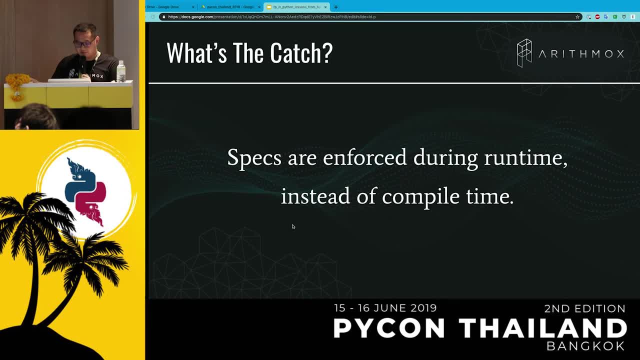 so sometimes it's it's it's more powerful right than static types. but there's a catch. all of these things run during runtime, not compile time, and really what that means is that you, uh the programmer, is responsible for testing, uh, once you've laid down all the spec infrastructure. 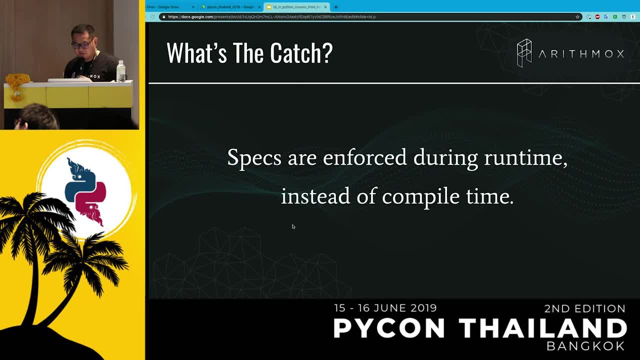 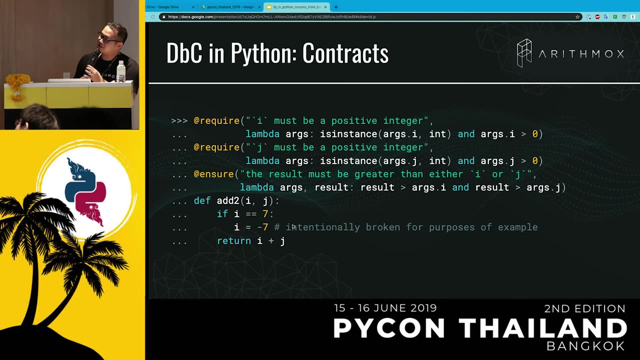 um, so uh, But Python doesn't have a static type checker anyway. Even if you use MyPy or Pyre, you can also combine it with this to get something powerful. Luckily there's this library called Contracts in Python. Unfortunately, it doesn't get many stars. 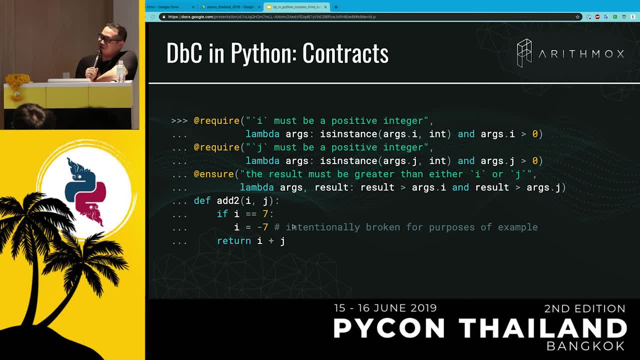 but do check it out and do give the author some stars, because I think it's amazing. It's very simple: Require is your preconditions, so it checks what your argument should look like, And ensure is a postcondition, so it checks how your result should look like. 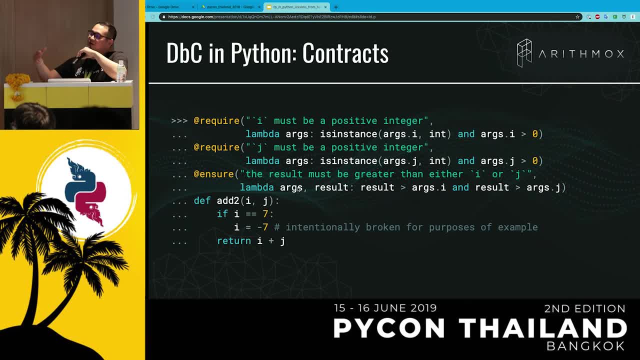 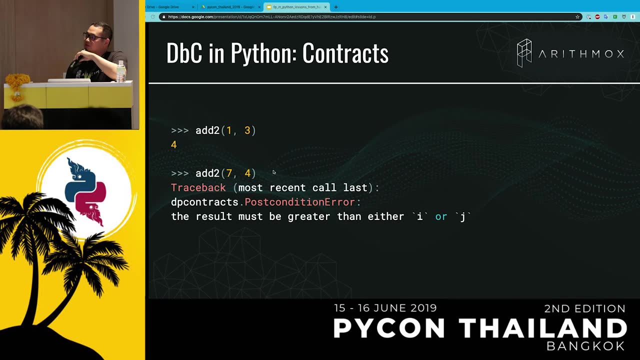 with or without in relation to the arguments. So this is a function that we intentionally break it. I took it off the readme directly And the idea is that you know, if you have a function that you want to break, if you do this, it works okay. 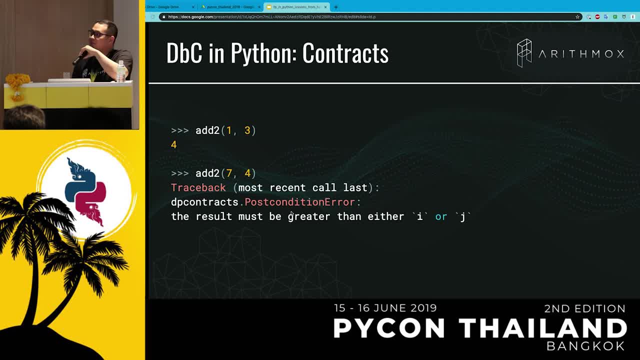 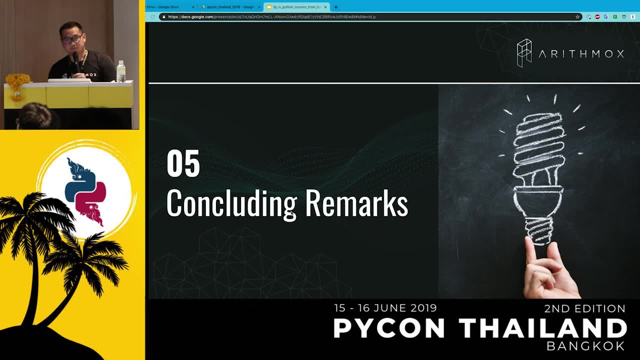 And if you do that, it gives you a nicer error, And you can combine this with property-based testing, which is really really nice. Anyway, that's Contracts. I want to quickly conclude. I think I'm running out of time. 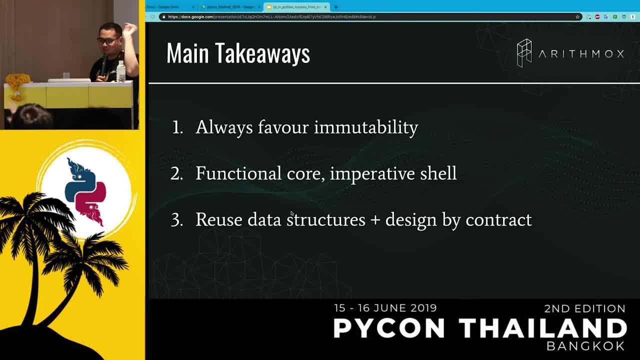 I've got 13 seconds. Always favor immutability. You don't have to go full Haskell. but if you don't do it unnecessarily, structure your code so that you know as much as possible. you want the code to be functional. 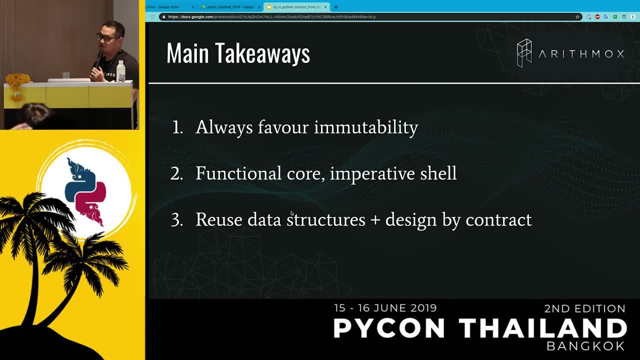 You know it's nice and you can compose nicely there, And the shell can be as messy as it is. I mean, yeah, within reason. So finally try using this technique. I can't say that I'm using it myself fully. 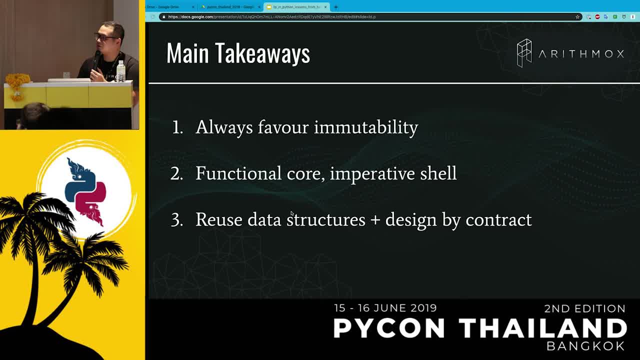 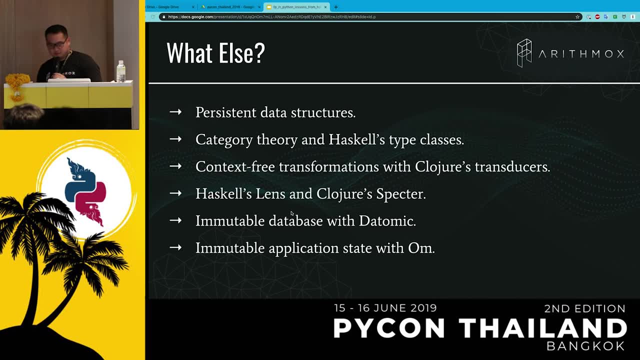 but I do want to. you know, it's something cool that I learned. I want to share this idea of designing by contract. You know when, when I- you know I pitched this talk. there's so much to talk about, right. 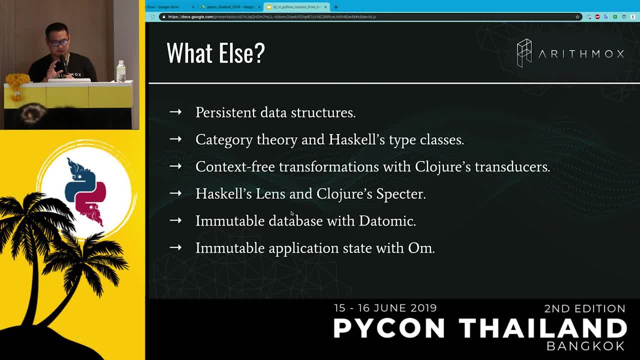 And really this functional programming is this: it's a goldmine of insights that you know you can pour back to Python And you know, you know. people say you know, you learn a new programming language and it makes you think slightly differently. 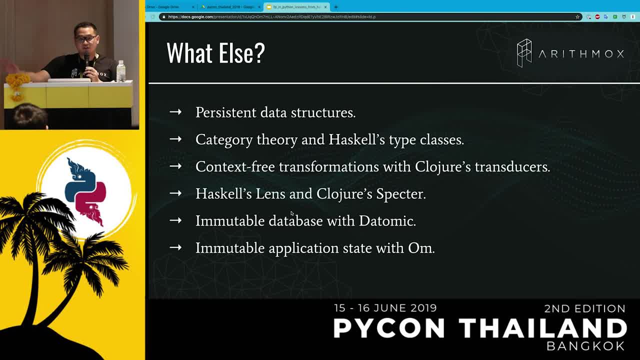 I think it's true. you know, with the condition that you learn a different language, It's a different family, right? If you learn Python, like Ruby is just yeah, it's not going to do anything for you. If you know Java and Haskell, you know Scala is you know? 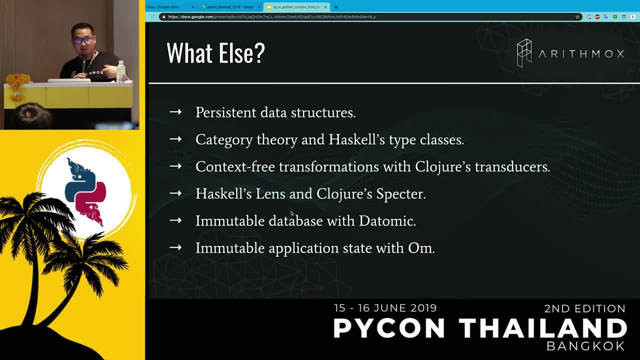 just maybe just the implicit: Learn Haskell, learn Clojure, Ada, Prolog, Idris, all these funky languages. you know, I, you know, I really believe that you do this, even though you're not going to use it in production. 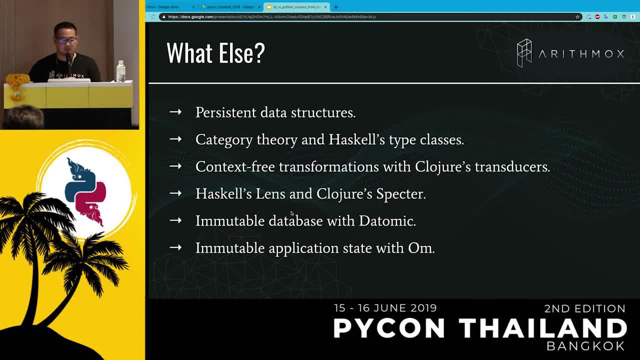 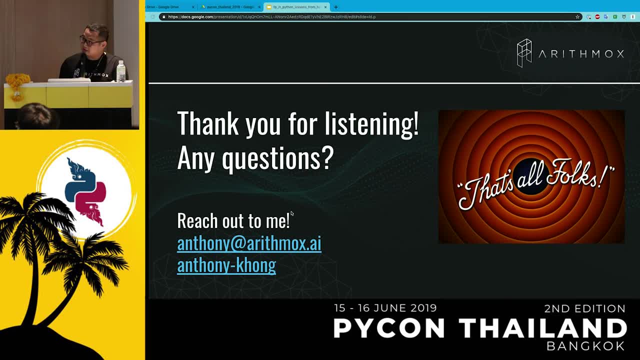 you're going to extract something and it's going to make you- it's going to make you- change the way you write your production language at work. I put some references there and that's it. Thank you for listening. Yeah, Maybe a short remark. 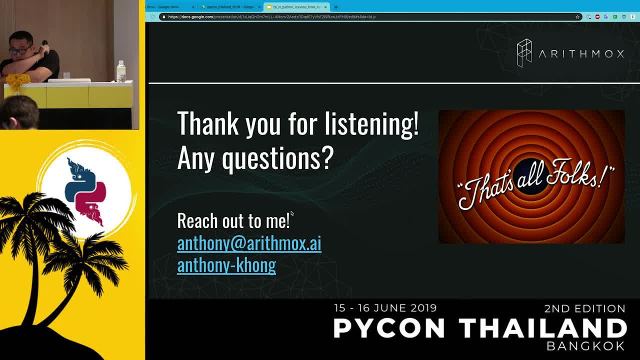 Yeah, So my name is Preshya from NETE. I wrote my entire thesis in Objective Camel. So the thing is, the category theory is really beautiful. But the thing is, when I switched to machine learning, I also used functional programming. 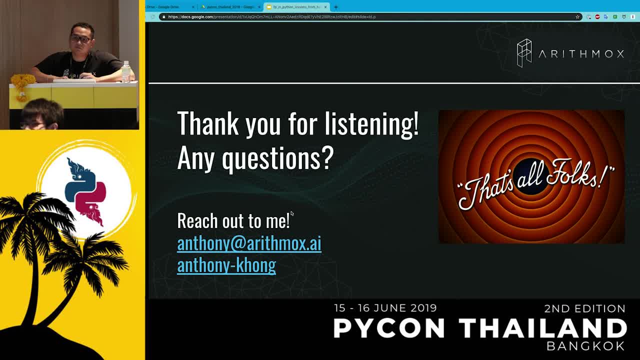 And it was such a pain, So I decided to move back to Python for that. And then, yeah, category theory in Python is like crappy. So are there any libraries that can combine the two worlds in one place so that they can stay on Python? 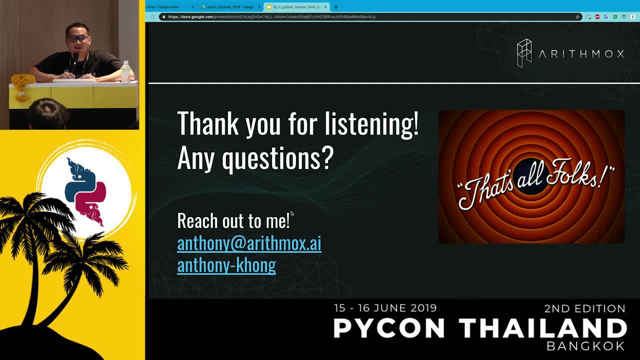 and then, yeah, use category theory. Okay, So I think there's a functional API for scikit-learn. I think that's out there, But I'm not necessarily recommending you to do that. It might not be production stable. 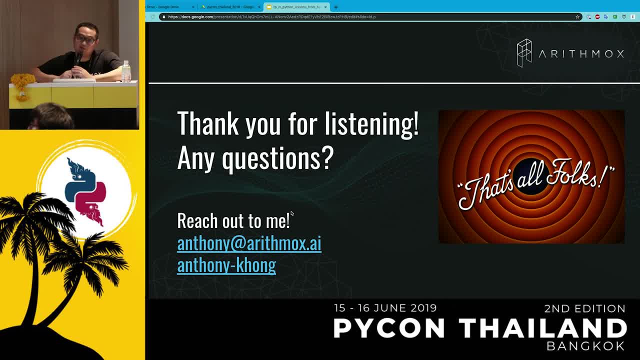 Look, there's a time and place for everything, right? Sometimes you know when you really need to do this. you have to do it. Yeah, You want to do the heavy lifting. You want to be standing on the shoulders of giants. 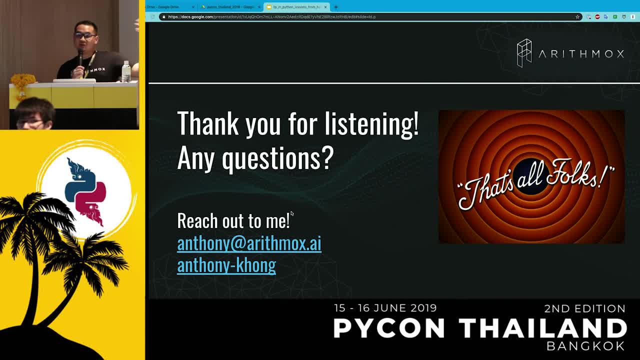 You want to have, you know, be using all the work that people put on NumPy, scikit-learn and Spark and TensorFlow and PyTorch. right, You want to do this And being a contrarian there. 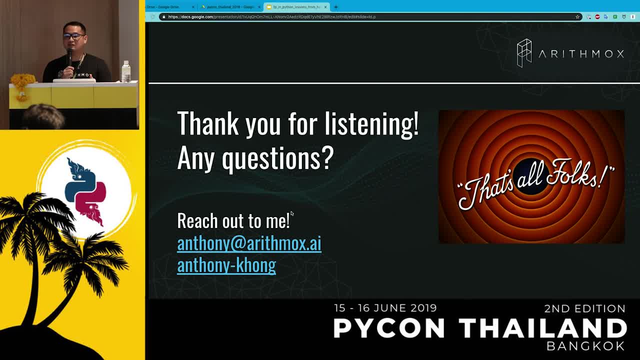 even doesn't matter how beautiful category theory is, how beautiful Haskell is, you know, I would still recommend staying within that ecosystem For machine learning. But you know, for some stuff, stupid stuff, like writing to an Excel, like I think it's a bit- 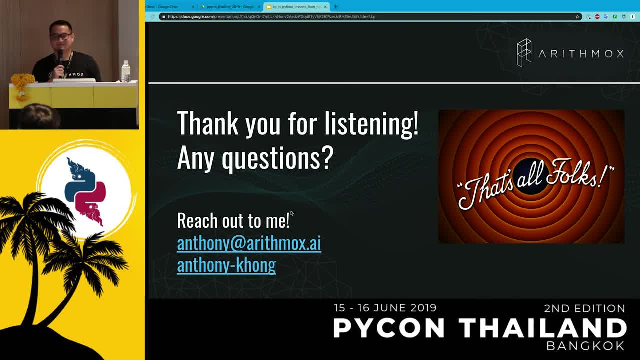 of fun to do this. Thank you, Yeah, Michael. Yeah, So you mentioned immutability. right, But generally bringing immutability into languages that were not explicitly made for it has certain tradeoffs. that is, that we kind of can still hear it because languages. 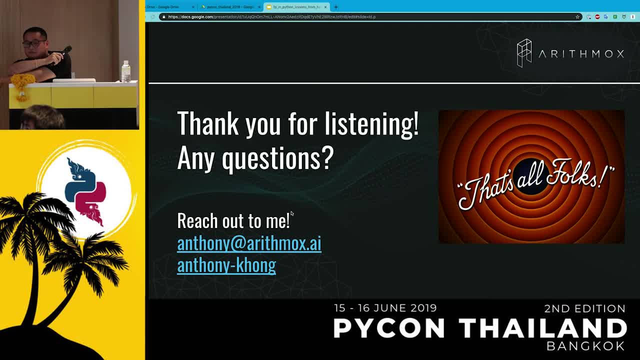 like Haskell and Clojure. we love them in languages which level to reuse as much of the data structure as possible and have pretty strong like copy and write semantics where only the piece of the data structure that changes actually gets changed. 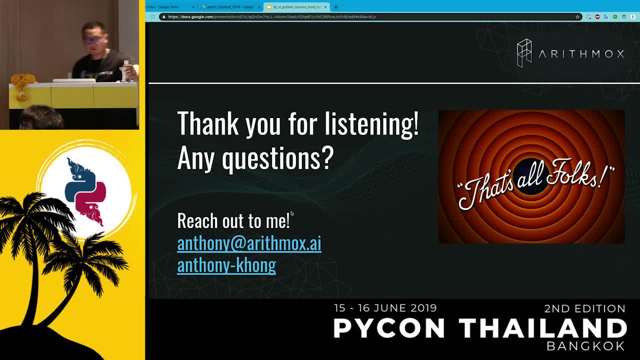 and everything else references the same memory because, well, it's immutable by default, so you know you don't have to change them. So like, for example, your Python workbook right That traded constant memory for linear memory for not really that much difference in expressiveness. 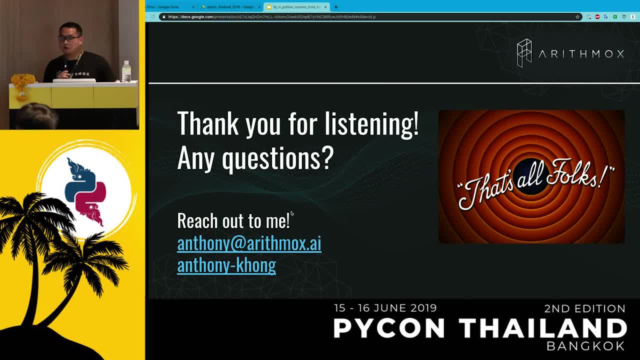 So do you feel those tradeoffs? Or is it in languages where, like, the language core itself does not actually really? because you said there's a right time and place, Yeah, So like, does immutability have a place in a language? 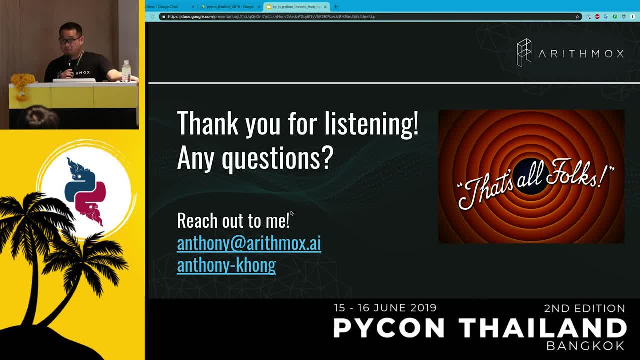 where it comes at a huge tradeoff in runtime memory. Yeah, of course, Like I can only say yes to that right. There isn't a good persistent data structure library in Python and maybe someone will write it someday and we can all use it. 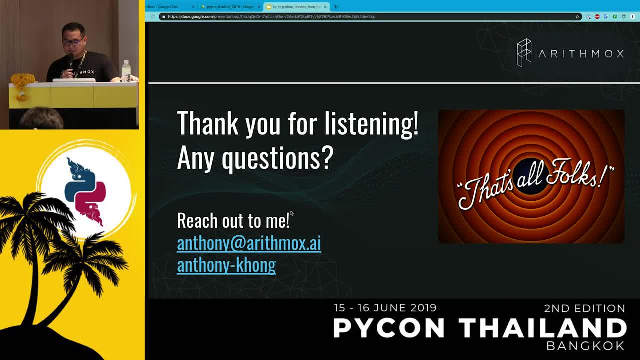 But I've always said: you know, I've always stressed that you know, in your own Python you try to make it as idiomatic as possible. As soon as that doesn't make sense, you stop, You don't do it. 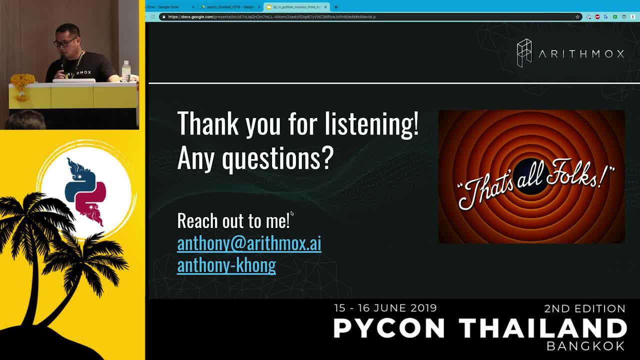 In the case of trading these. so performance considerations, yeah, I mean again, that's pragmatism, right, Like if you're going to write like a billion cells, don't do that. If you're going to write 1,000,. 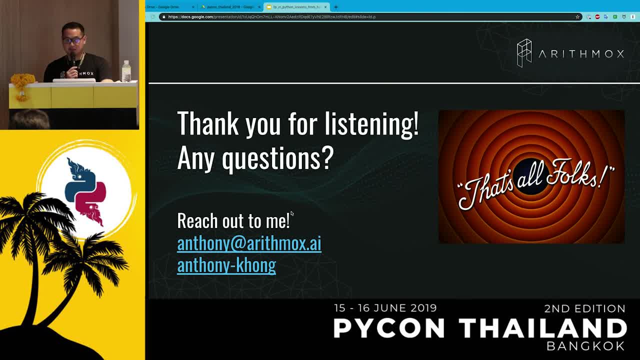 whatever you know. So, yeah, there's this. you know I preface this with all the pragmatism that there is, There's a time and place for these. I find these things really nice to express and yeah. 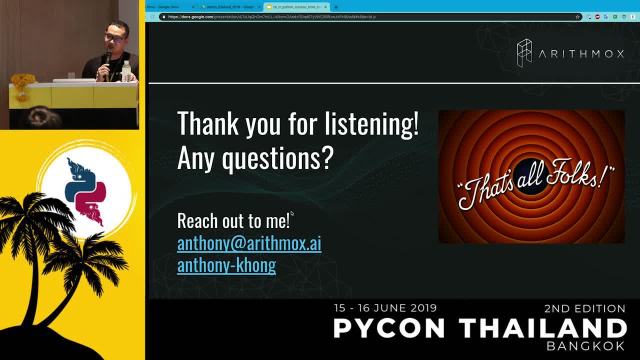 use it in the right time And I would disagree with you that it's not as expressive. You know you don't get as much expressivity if that makes sense. But I think I think maybe we can chat a little bit. 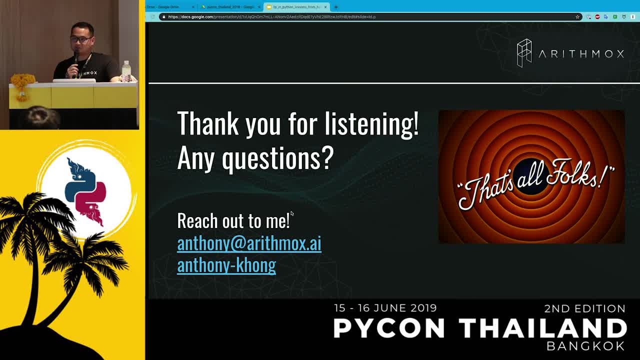 You could have started to call it 10, then the other thing wouldn't have been as contrived as the example. So, yeah, look, I took that example directly from the thing, right? So that's meant to be idiomatic way of you to use that library. 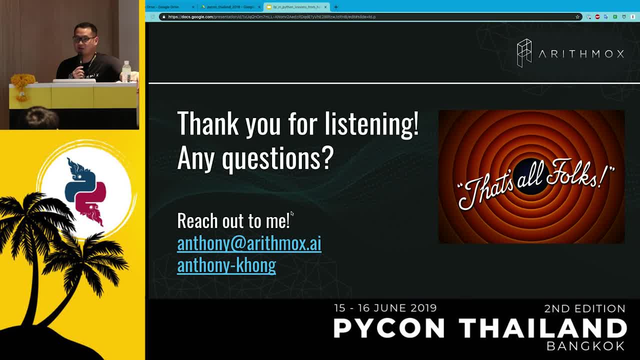 which is, yeah, not fantastic in my opinion. I think that's one more right, So I can use my background, but you're over the top. I'm Colin and I used to do a language program, And these languages are very practical languages. 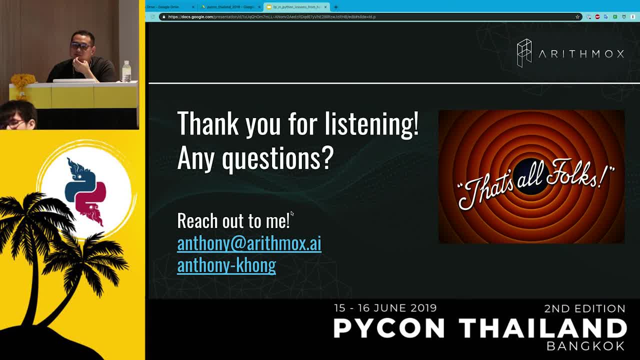 And since Java 8 and the beginning of the problem they start to add functional on top of the base of the language, But they're still at the base of the language. So I really like what you said about kind of encapsulating your mutability. 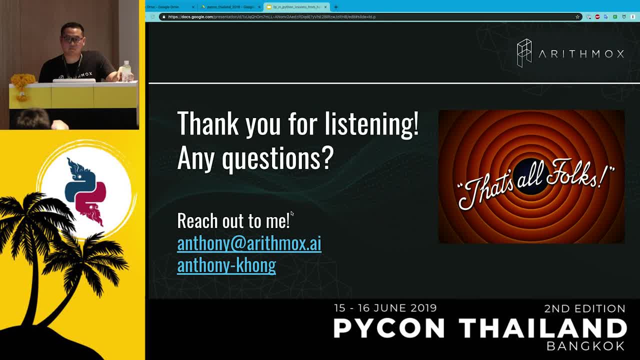 like kind of playing with your mutability. so it's still there in the performance, But then when you're building off the back of it, you're not. You're not exposed to the root for it. Right, You mentioned at the start there were no logs. 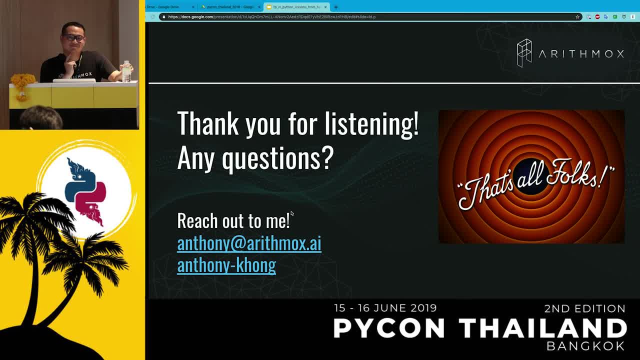 Yeah, So when I'm writing Java and Kotlin nowadays I'm using the kind of functional APIs: lots of streams, lots of sequences, So it's kind of a list of map operations. I'm not so familiar with Python. Is there some way of getting back kind of a bit of that? 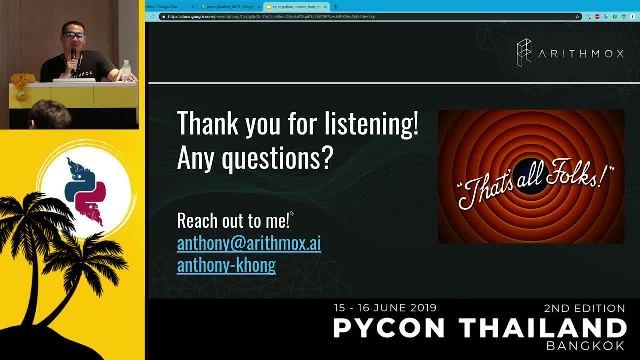 Yeah, that's a good question. Like I tried it myself, I hated the way. I hated the way it looks. So, you know, when you're composing all these functions together, it's, you know, especially higher-order functions. 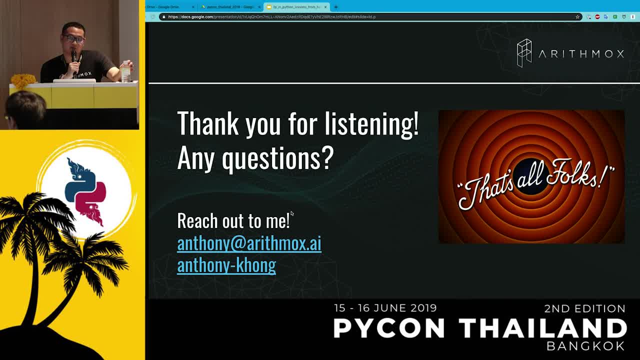 One. you need to do. a lot of imports Like partial is not built in, Right Reduce is not built in anymore. It's a hassle. There is a few things out there. There's a library called Tools with a Z, or SciTools. 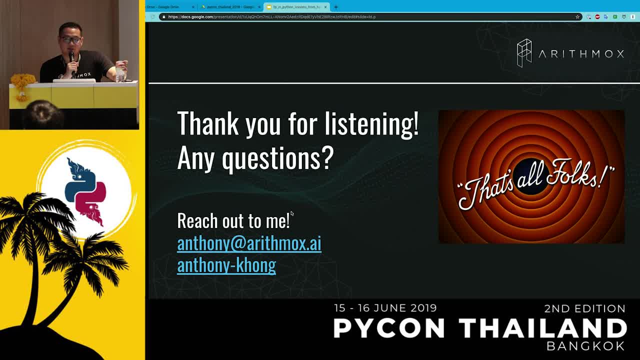 which is like a rewrite of Tools with Python And some constructs there are interesting. You get the pipe and all that, which is quite nice, And there's also a Python transpiler called Coconut. That's also very interesting, though it seems to be a bit bloated nowadays. 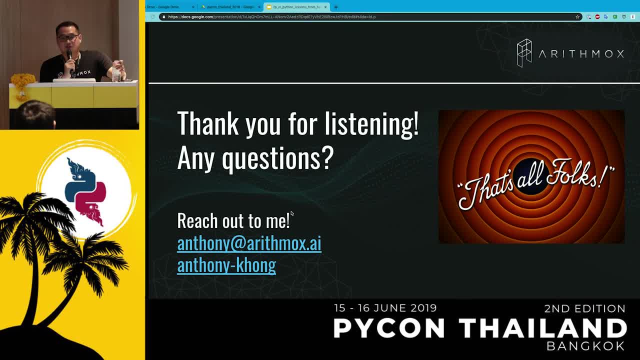 But people are using it in production so that's quite interesting. So I guess have a look at these. But again, like I wouldn't force the issue if it looks terrible,